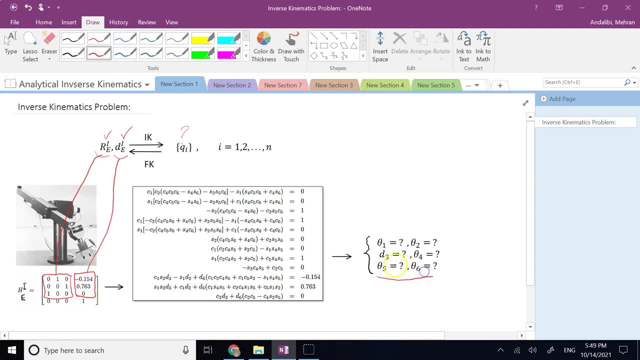 matter of fact is, I only need to find what Six unknowns, theta one, theta two, theta four, five and six and D three, which is the value of this prismatic joint. So, first of all, I have 12 equations. 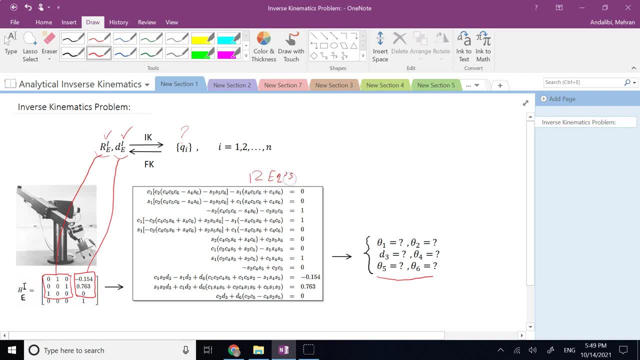 Second of all, and six unknowns, And that means my system of equations, is what Is over constraint? right? So my system is over constraint, And you might say, well, is there then an accurate solution? Because typically, when your system is over constraint, that means you can at best find what, At least a square solution, or 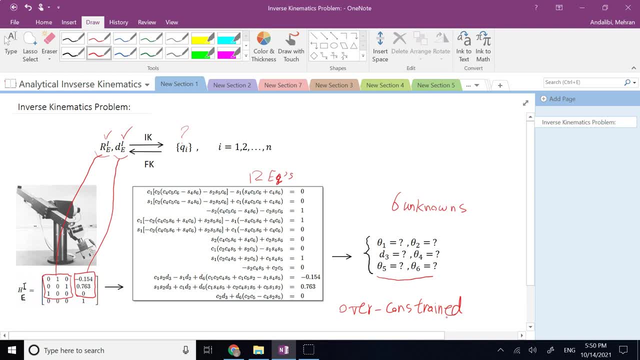 something, an approximate solution. But the matter of fact is, in this case there are what. There are six constraints here. What are those constraints? Well, those are the constraints for the rotation matrix. If you remember, each column of the rotation matrix has a magnitude of 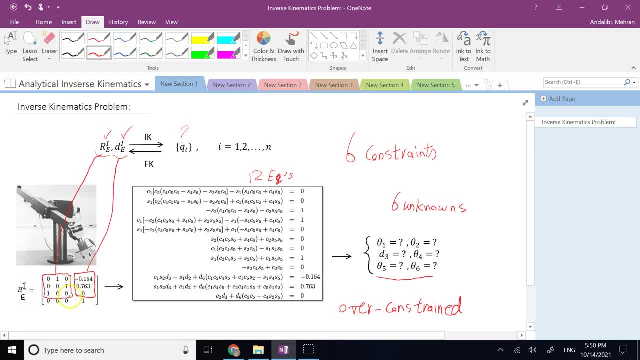 one, and then each column is perpendicular to the rest of the columns. So column one dot product with column two, column one dot product with column three, column two dot product with column three, they're all zero, And magnitude of column one is the same as magnitude. Column two is the same as. 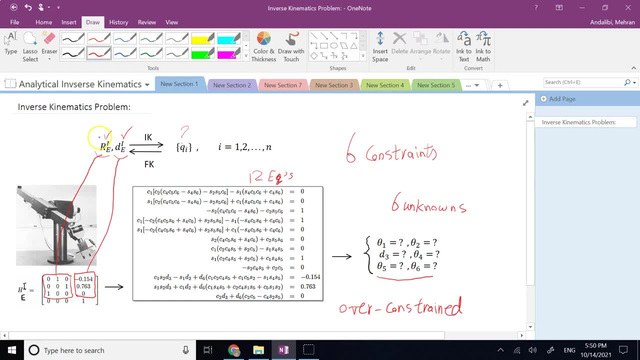 magnitude Column three equals one. So those are those six constraints coming from this rotation matrix. So what you need to solve for are 12 equations and six unknowns, but there are six constraints which are in terms of all of these variables, And that makes the solution of that. 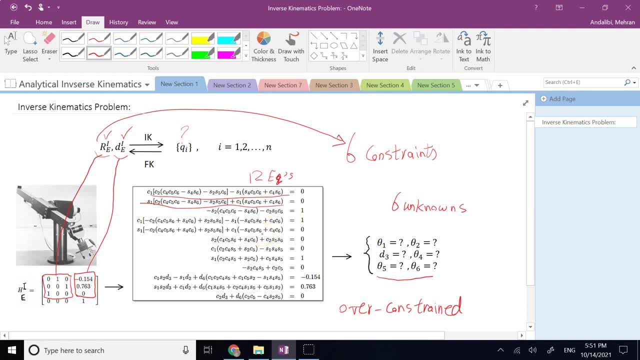 almost impossible If you don't have a spherical wrist here, which in this case you do. but if you don't have a spherical wrist and the robot has six degrees of freedom, or sometimes more, then in general the analytical system is not going to be able to solve that problem. So what you need to 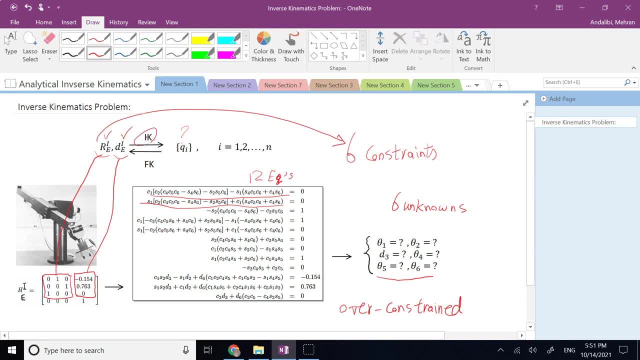 do is: you need to solve that problem. So what you need to do is you need to solve that problem, So you need to solve that problem. So the quadratic solution of inverse kinematics problem is not always possible. For some scenarios it is possible. For some scenarios it is not, And even 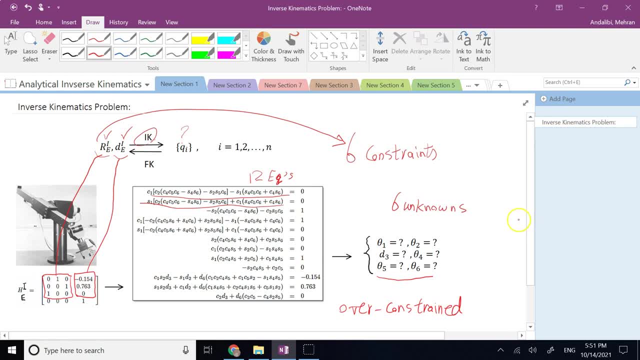 when it is possible. it's not really a trivial thing. So that's one problem. The other problem we have is the multitude of solutions. If you remember, if I give you the variables theta one, theta two, theta four, five, six and d three and the geometry, you're going to get the 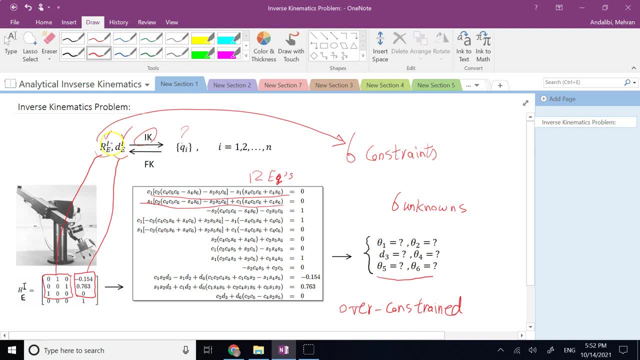 geometry of the robots, then there is what One unique solution that you will find for the rotation matrix and the position vector. As long as the values I give you for the six variables are within their mechanical limits, then there is always what A unique solution to the forward. 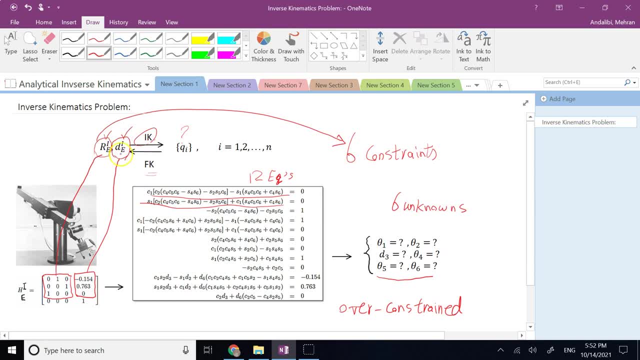 kinematics problem. On the other hand, if I give you the inverse problem and I ask for joint variables, we can see there are different scenarios. There are scenarios where the inverse kinematics can have no solution. There are scenarios where there is no solution at all for 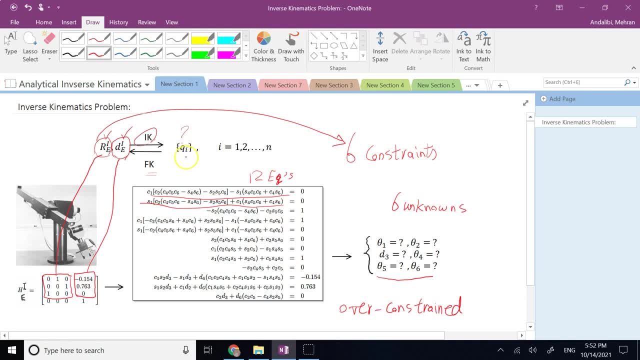 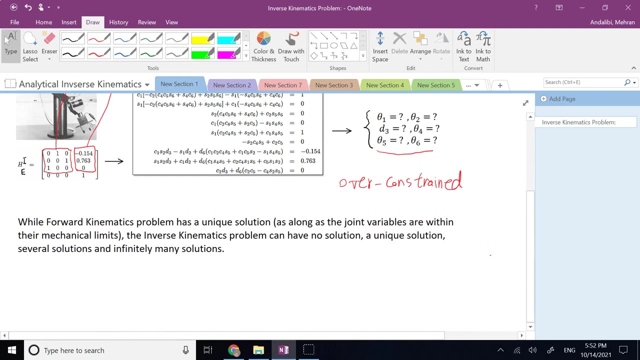 queues. There are scenarios that there is a unique solution, There are scenarios that there are several solutions And there are scenarios that there are infinitely many solutions. okay, So that's another big important difference between forward and inverse kinematics. Inverse kinematics. 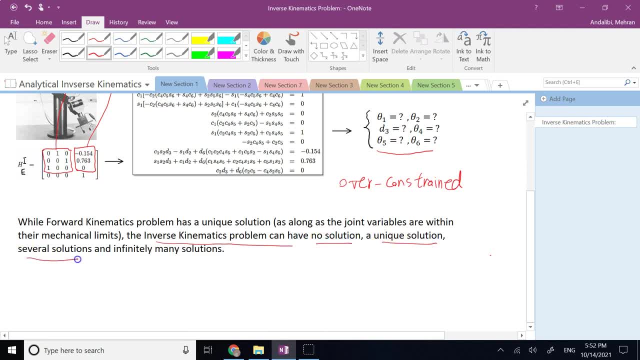 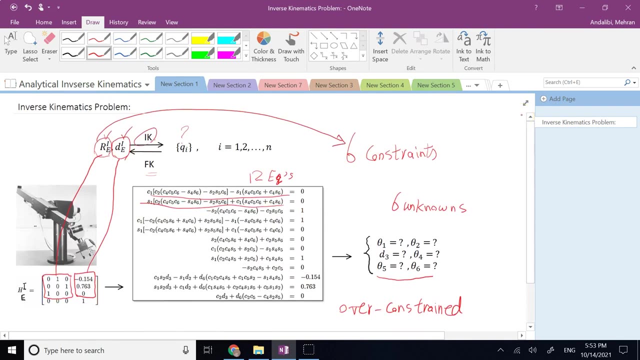 can have no solution, unique solution, several solutions or infinitely many solutions. So again, forward has only a unique solution as long as the joint variables are within the mechanical limits, And I'll show you all of these scenarios here through even simple examples. So in general, 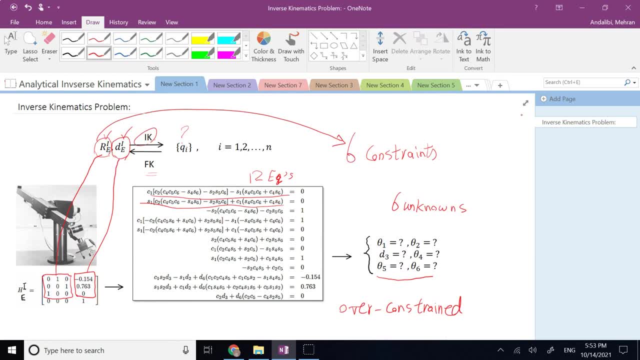 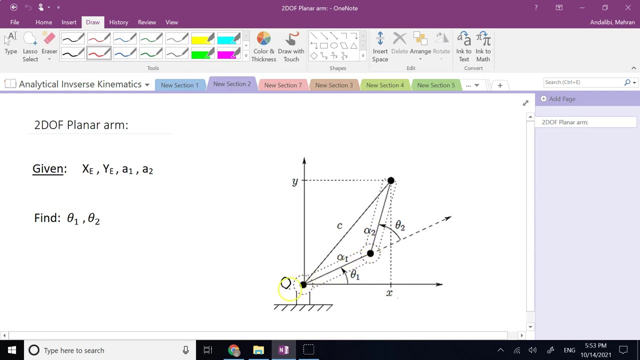 if you want to put it in a nutshell, inverse kinematics problem is much more difficult than forward kinematics. Okay, So to start explaining all of this, we start with the kind of the simplest robot that we know, The two degree of freedom, planar arm right. So we have two members here with sizes of A1 and A2.. 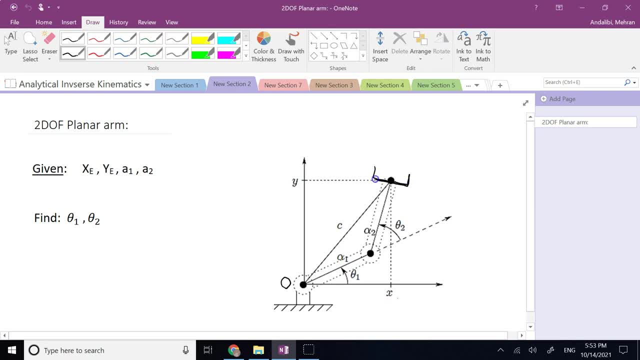 And let's say: here we attach an end effector, here gripper, let's say: And the positions of the end effector in base, X of E in zero and Y of E in zero, these two guys are given to me, As well as. 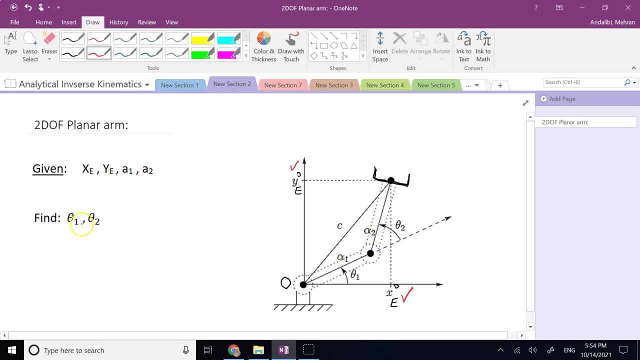 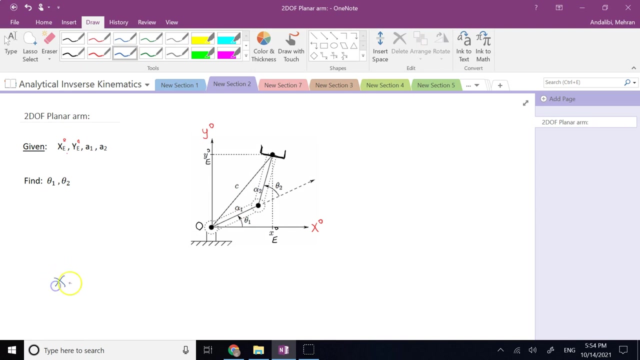 what A1 and A2.. Then the goal is to find the angles of the two members, theta one and theta two, correct. So that is your analytic inverse kinematics. So let's see how we can potentially find solutions here. So if we write our forward equations, forward kinematics equations, then you know that X of 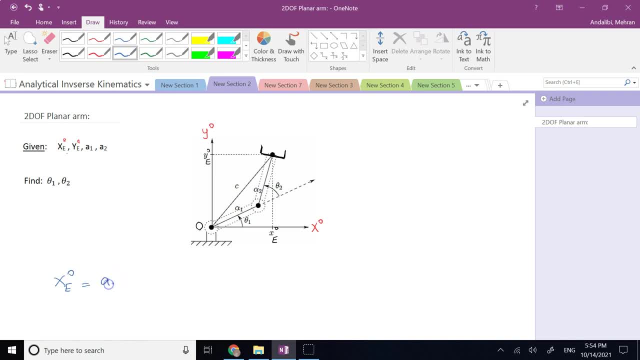 base is equal to A1 times C1 plus A2 times C12.. As you remember, C1 is cosine of one theta one, C12 is cosine of theta one plus theta two And similarly Y of end effector in base is: 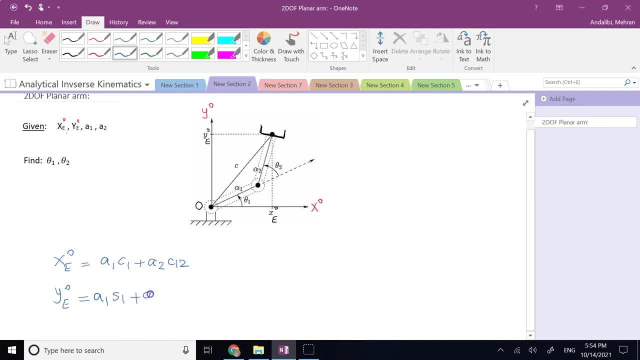 A1, S1 plus A2, S12.. Okay, So clearly you have two equations and two unknowns. The equations are linear in terms of the unknowns, But in this case, because the robot is not very complicated, we can. 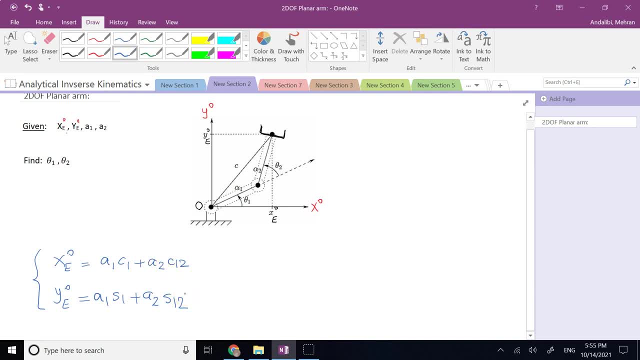 find solutions both using geometrical approach and also the direct mathematical approach, pure mathematical, without any geometrical interpretation. First geometric approach. So in geometric approach, here I'm going to name origin O. I'm going to name this first joint A. 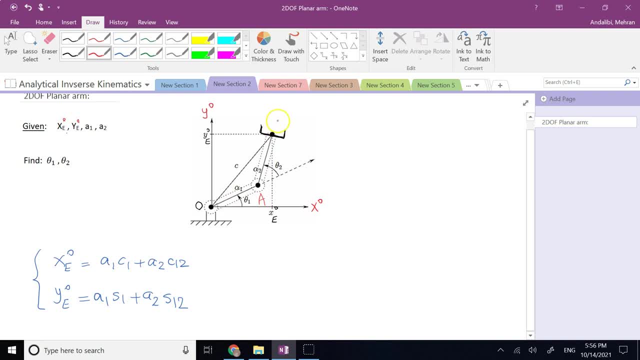 Or second joint really, And the end effector E. I'm also going to call this point where this X of E is happening, this point. if you don't mind, I would call that point C And I also need to draw a. 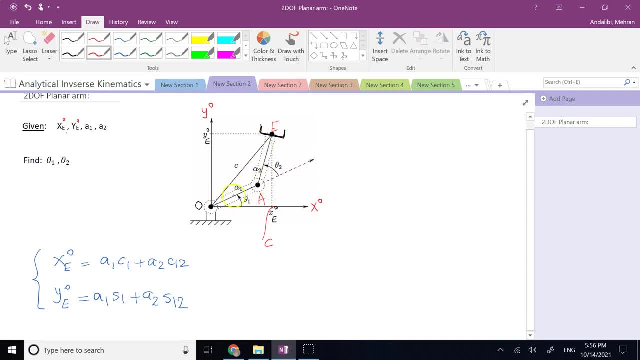 perpendicular from E to the line of action for member one. So from here I draw a perpendicular line, this line here, And the bottom point of this I call it D. So I have A, O, A, E, C and D. Good, First question is, if I want to find this angle here, this one, I can. 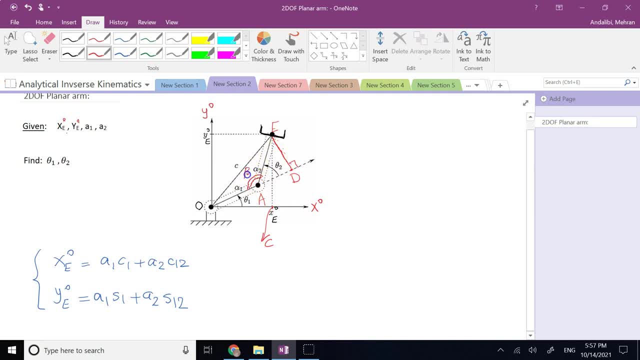 call it whatever you want. Maybe I call it angle beta. So how do I find angle beta? Well, angle beta is in the triangle O, E, A. And this triangle, two sides of it, are A1 and A2. And this side, which I called C, 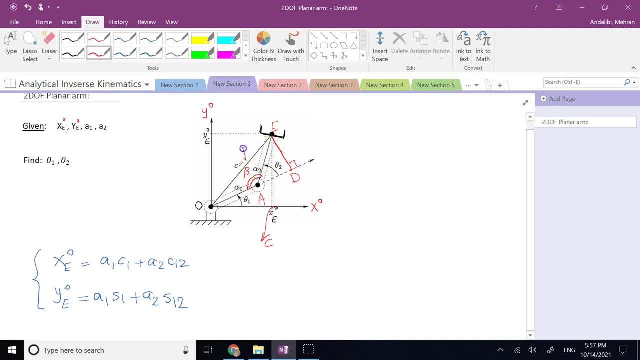 the hypotenuse is clearly what It is: the square root of X of end effector squared plus what Y of End effector squared right. It's the hypotenuse of the triangle O, E, C. So clearly I can, let me write it. 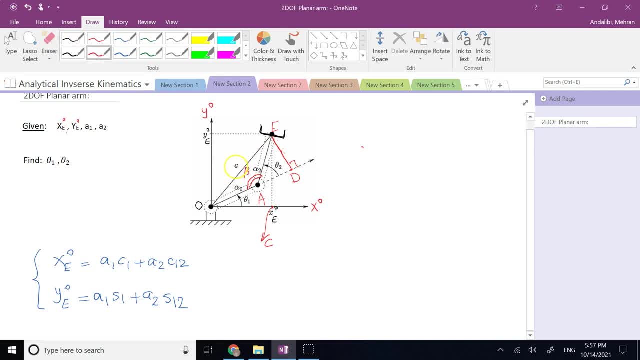 bigger a little bit. So this guy here is the square root of X of end effector in base squared, plus Y of the end effector, Y of the end effector in base squared Right. So you have this triangle. This is A1.. This is A2.. This angle is beta. 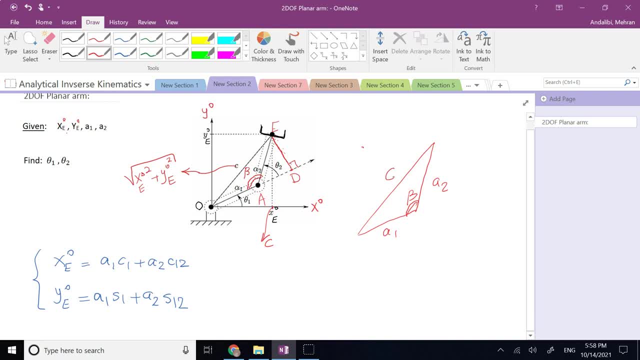 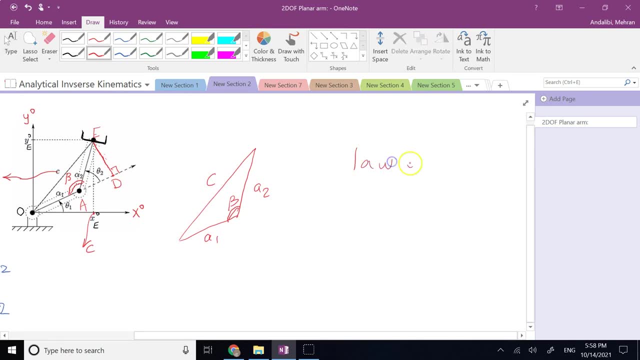 And this side is that C. How can I find C? Using the laws of cosine or law of cosine? Law of cosine says what It says. C squared equals A1 squared plus A2. squared minus 2A1A2. cosine of beta. 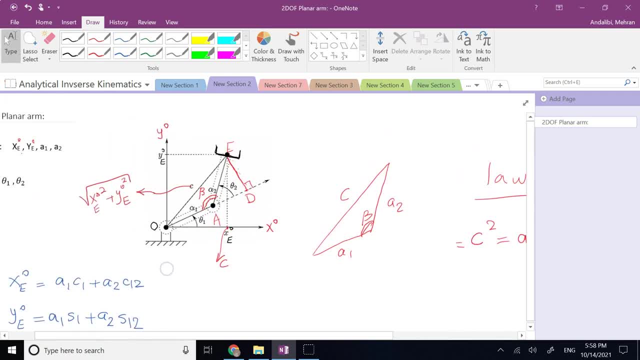 And you know that C squared, based on what we had, is going to be that whole thing where the square root is taken out. So it's going to be the whole thing where the square root is taken out. So it's going to be the whole thing where the square root is taken out. 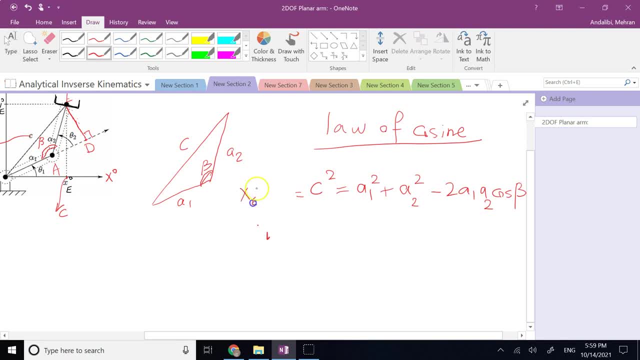 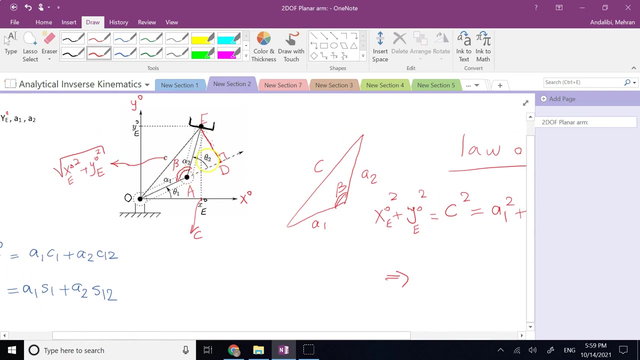 So it is going to be X of end effector in base squared plus Y of the end effector in base squared, Correct, So from here I can clearly find what I can find: cosine of beta. But you know, beta is related to theta 2.. Clearly beta plus theta 2 is what 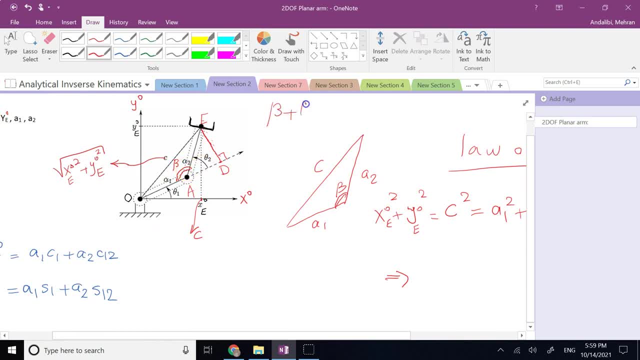 180 degrees, right, So beta plus theta. So when two angles are such that some of them is 180, you know that cosine of 1 is negative of cosine of the other. So instead of cosine beta I can use negative cosine theta 2, correct? 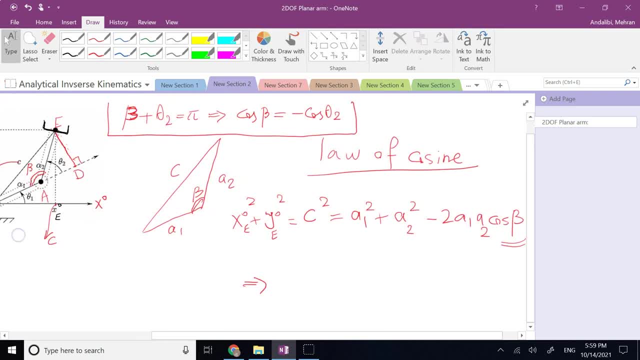 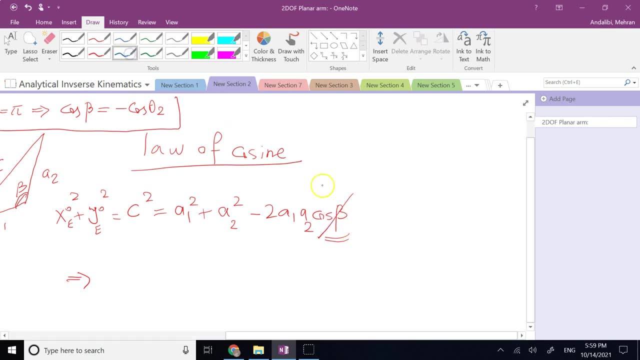 This we know from trigonometry. So if I plug it up here, then it is going to be, as I said, negative cosine. This we know from trigonometry. So if I plug it up here, then it is going to be, as I said, negative cosine of theta 2.. 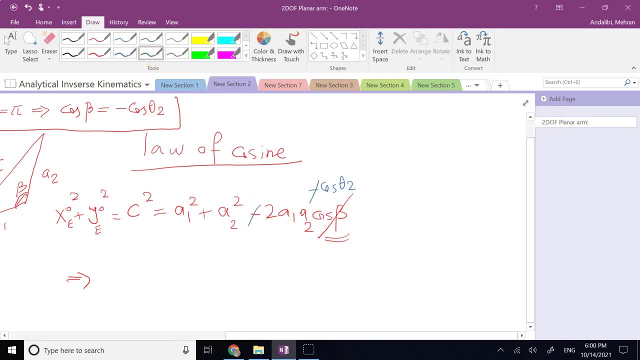 And then these two negatives would cancel out. And so from here I can directly find cosine of theta 2, which is going to be X of the end effector in base, squared plus Y of the end effector in base, squared minus A1, squared minus A2, squared then divided by 2A1A2.. 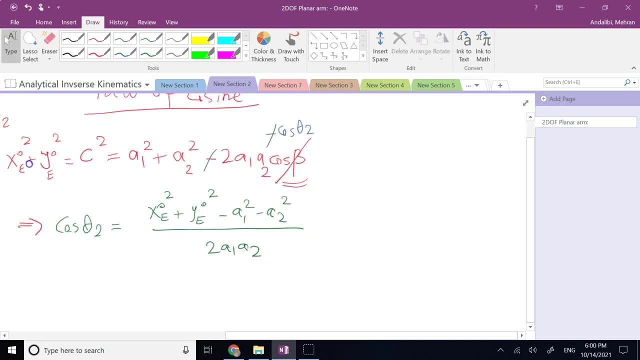 Okay, And this formula can give me cosine of theta 2.. And now you might say: well, I take a cosine inverse from both sides and that gives me theta 2, one of the two unknowns. Yes, you can do that. 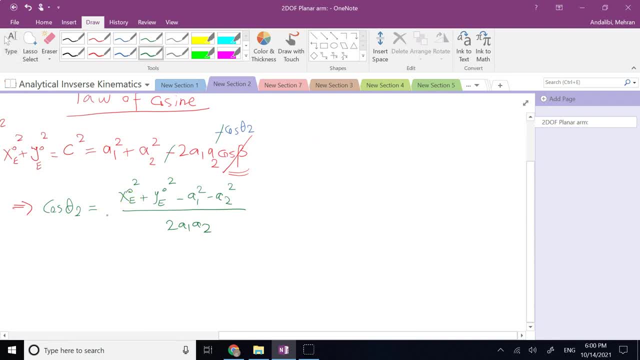 But the problem with the arc cosine function or the regular arc tangent function is they are not quadrant corrected. Okay, So what we do typically in robotics, instead of using the regular arc tangent, which only takes the ratio of Y over A1, or X, or arc cosine, we use this quadrant corrected function, which we call arc tangent 2,. 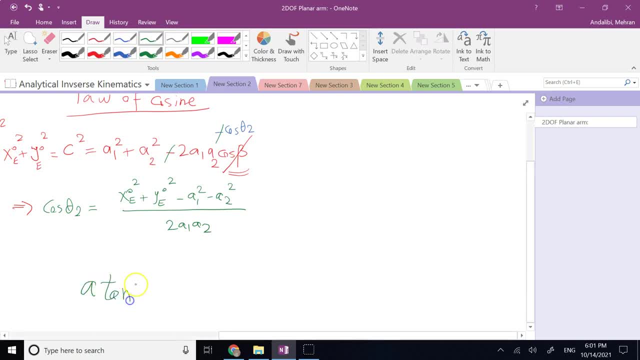 which you know. there is this function in MATLAB, arc tangent 2, which it takes both Y and X, Instead of the regular arc tangent that takes what Y over X. So for a regular arc tangent function the ratio matters, So if both of them are positive, 1 or negative, 1,. 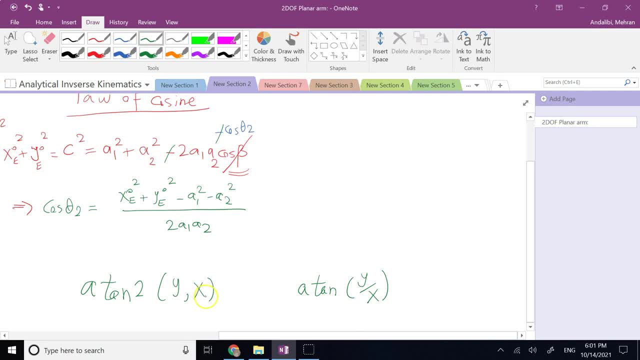 the ratio is going to be 1, while for this one positive, positive 1 means it is in the first quadrant, negative, negative 1 means it is in the third quadrant. Okay, So this arc tangent is not only more accurate than the regular arc tangent, 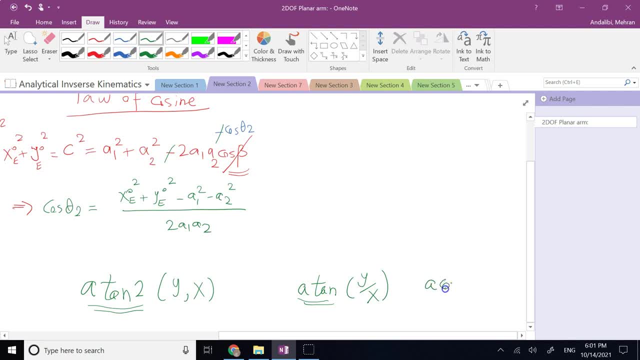 it is more accurate than arc cosine. Okay, Which is basically X over R, Because, again for this one, as long as X is positive, it does not care right Whether it is in what First quadrant or the fourth quadrant. 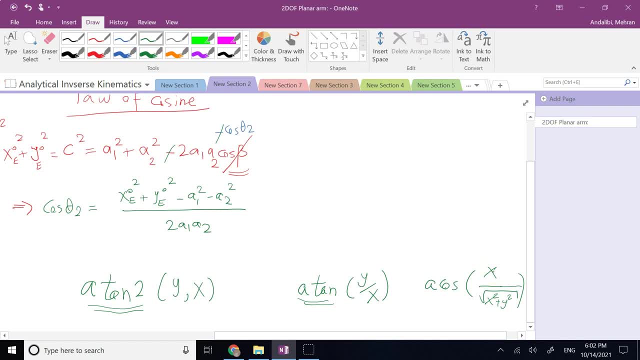 For both of them, X is positive, or if it's negative again, it could be in the second quadrant or the third quadrant. It only cares about sine of X, because this square root is always positive. So instead of regular, as I said, arc functions, we use arc tangent 2.. 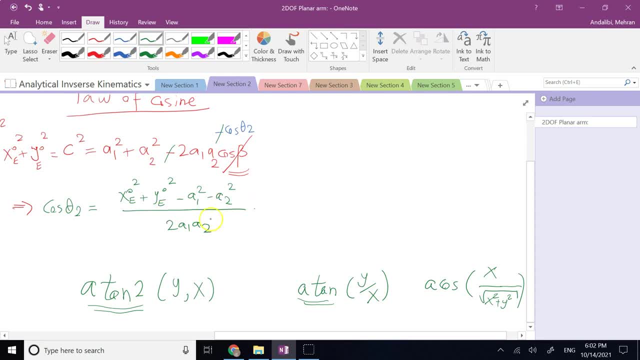 How Well, from here. So from here, if I call this whole ratio, which is just a single number, right, Because X and Y are numbers, A1 and A2 are numbers, If I call this whole ratio just number D. 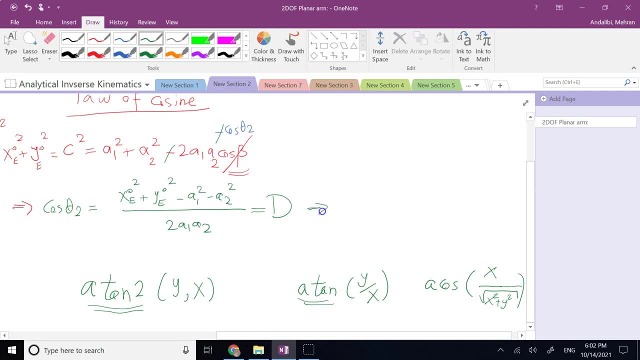 and that D is equal to cosine of theta, then from here sine of theta 2 is going to be plus or minus square root of 1 minus D squared or 1 minus cosine squared. So now I have both. So I have sine of theta 2, and I also have what 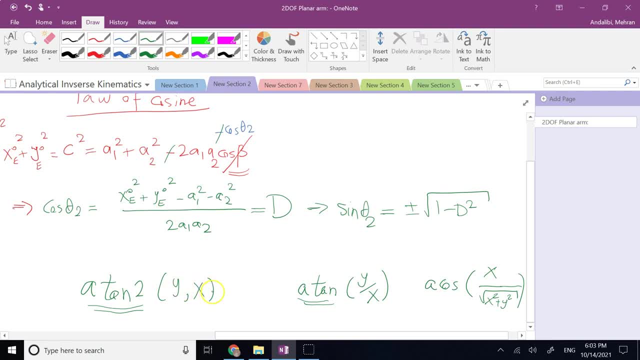 Cosine of theta 2, which corresponds to what? Y and X. Therefore, I use what I use these two things I found for sine and cosine, and then I find theta 2 through arc tangent. So theta 2 is going to be arc tangent 2 of what? 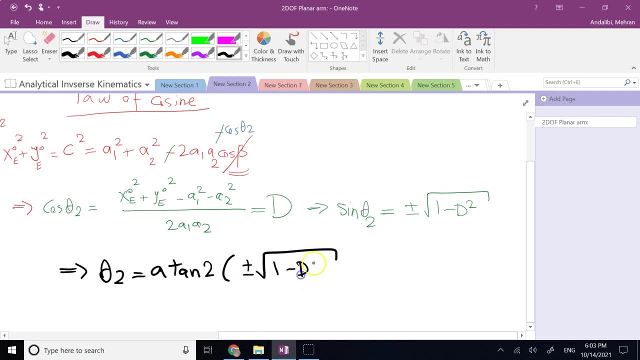 Plus and minus square root, 1 minus D squared, which is sine of theta 2.. And then the D itself, which is cosine of theta 2, where D is this ratio here. Okay, so that is ratio and this is what. 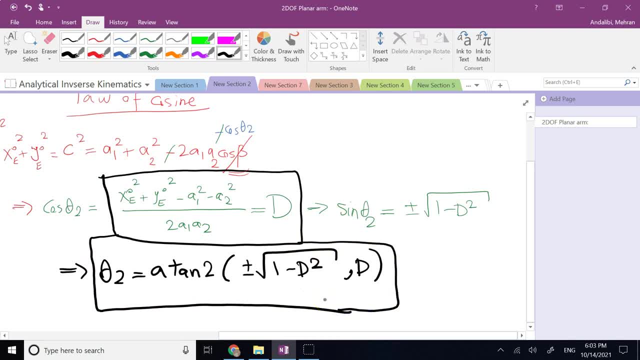 D. So this is the formula I use to calculate what Theta 2.. And clearly this formula tells you that there are two answers for theta 2.. One is for positive square root, The other one is for negative square root, And I'll show you. 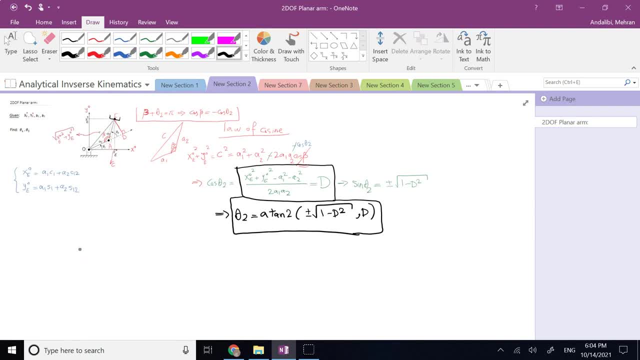 We are done with the solution. I'll go back and show you what's the meaning of positive and negative. Okay, But clearly you see that your inverse solution can have more than one answer. It can have two answers as far as just theta 2 so far. 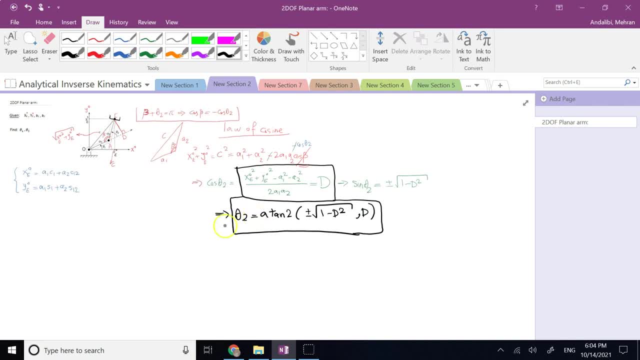 So good, I got my theta 2.. Now what? Now you might say, well, plug that theta 2 back here in one of these and find theta 1.. Yes, but that I can do with a mathematical approach. As I said, I want to find theta 1 and 2 with geometry. 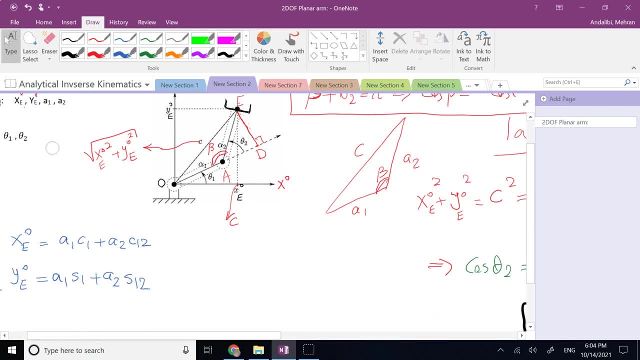 So then you might say: well, how do you find it with geometry? This is what I do. So here I would call this angle, this big angle, here this one, This angle, you can give it again any name. 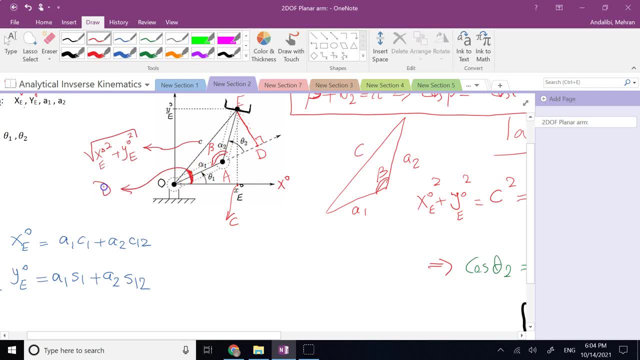 Maybe this angle. I call it gamma, You don't mind, Right? So that angle is gamma, And I also have this smaller angle, This one And this angle again. I can call it something else. Let's say for example here: maybe delta. 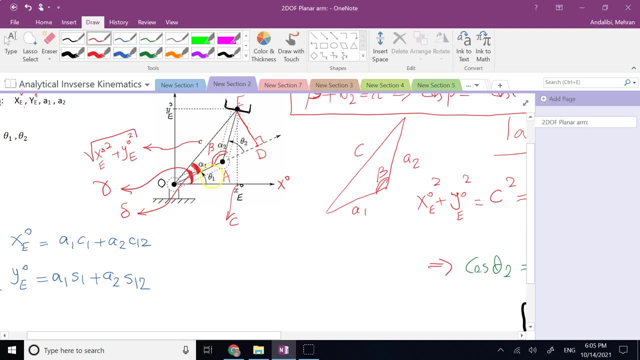 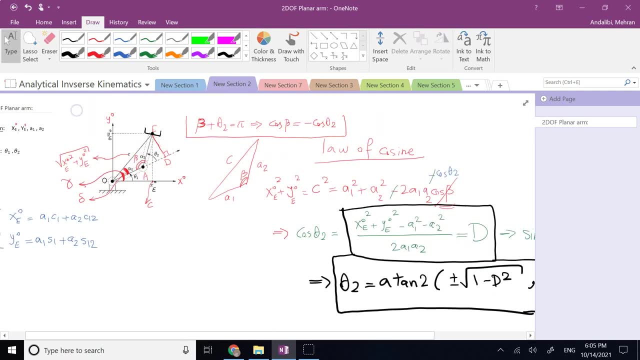 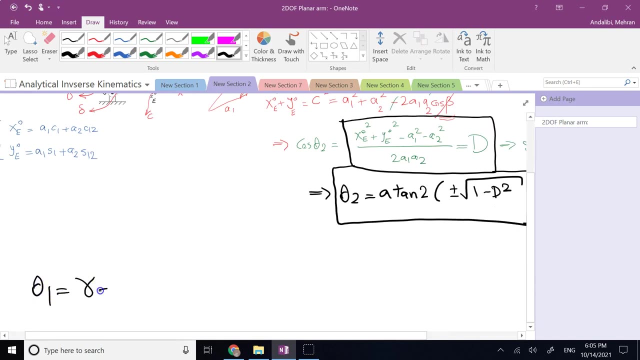 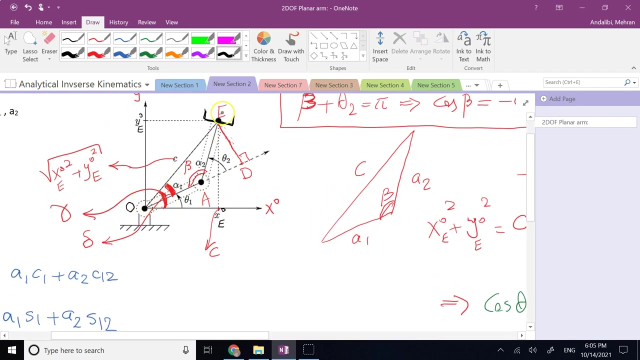 So gamma minus delta is clearly what Theta 1.. So theta 1 is gamma minus what Delta, Right? So if I want to write it somewhere, then clearly your theta 1 is gamma minus delta. What is gamma? Well, gamma is in the big triangle OEC. 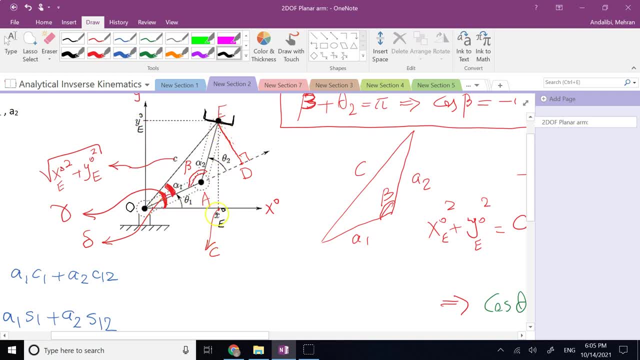 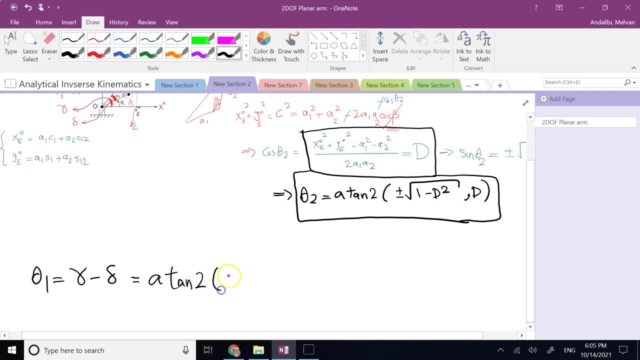 The y of it is y of the end effector, The x of it is x of the end effector. So I can use that same arctangent 2 function I just told you and pass to it y of the end effector and x of the end effector. 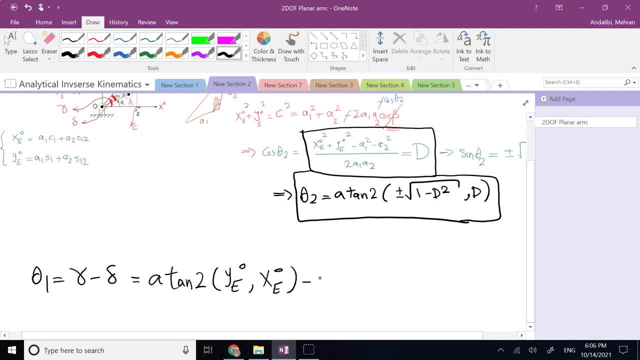 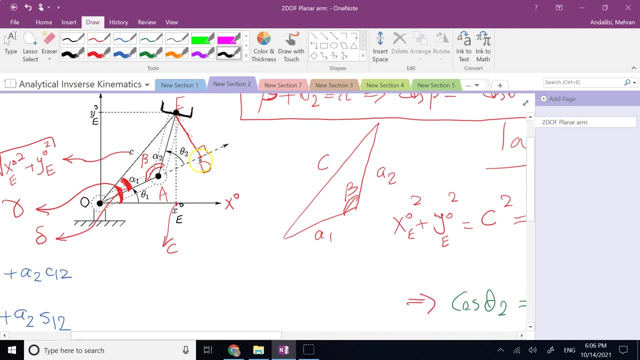 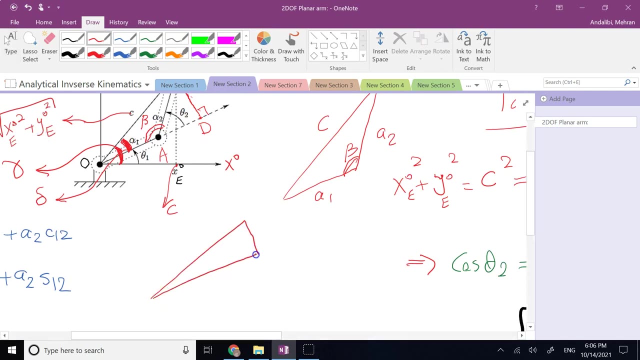 And that will give me back gamma Minus. What is delta For delta? I use this triangle OED. If I draw that OED for you here, it has this part of it A1.. This part of it is A2.. 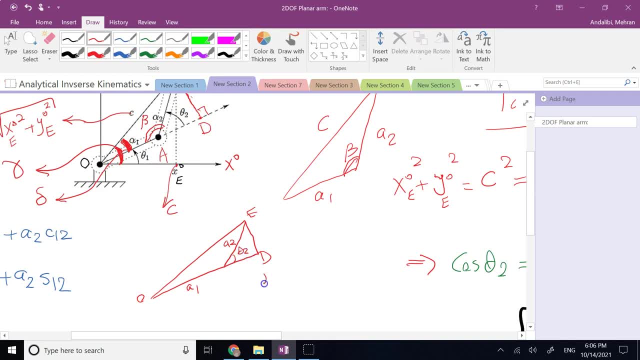 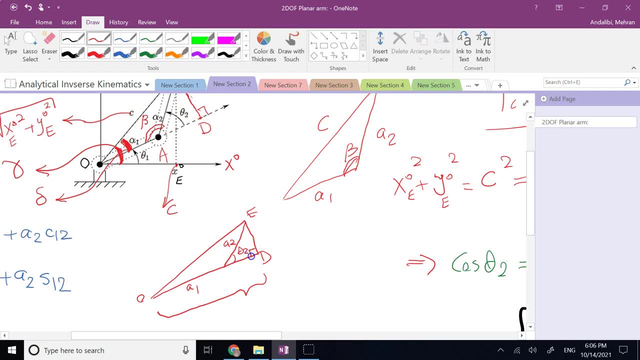 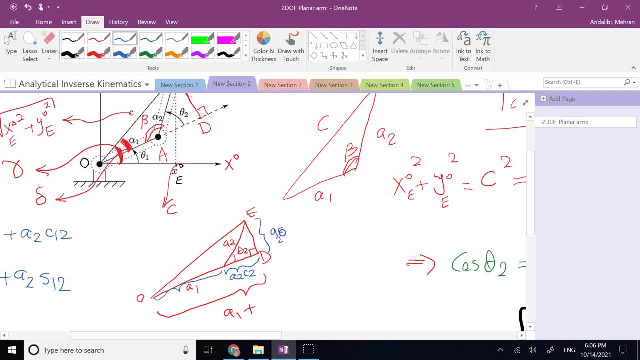 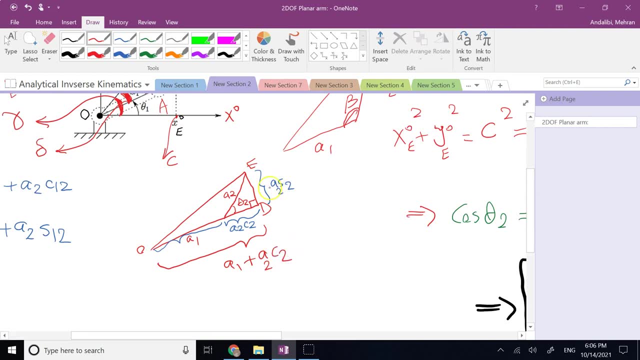 And this opposite to it is A2 sine theta 2.. Okay, So clearly the whole adjacent is A1 plus A2 cosine theta 2.. Okay, and the one opposite to it is a2 sine theta two. so if i pass those two arguments to the 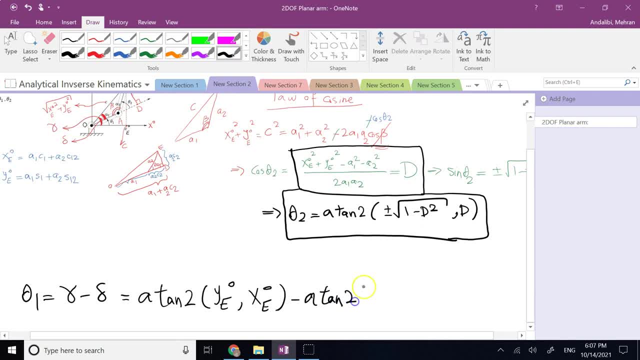 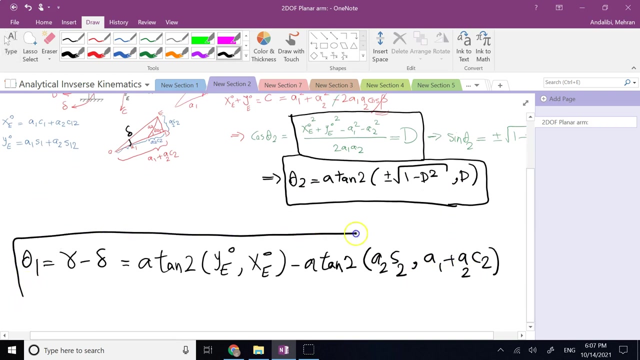 r tangent two function right. so a2 sine, theta 2 and a1 plus a2 cosine, theta 2. that should definitely give me that angle delta and that's what you see here. and guess what? i already calculated theta 2 in the previous step, so i just need to plug it into the sine and cosine and this one gives me what theta 1. 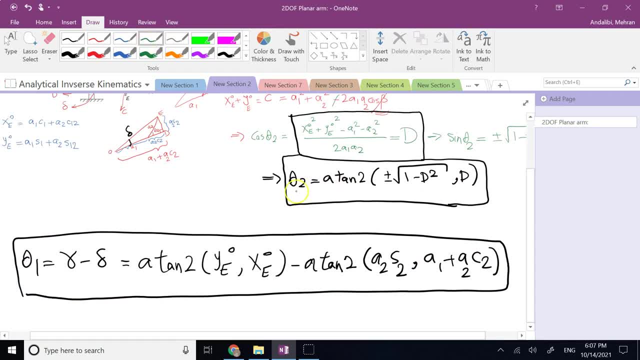 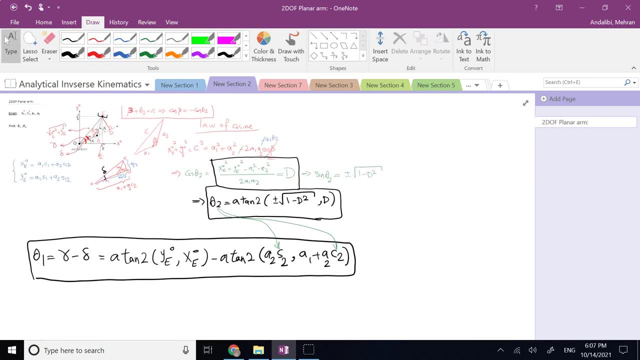 again, this theta 2, the sine and the cosine of it, should be used here. done, and these are my solutions: theta 1 and theta 2. so if i pass those two arguments to the r tangent two function, for each theta 2 there will be a corresponding theta 1, of course. so in general there are two. 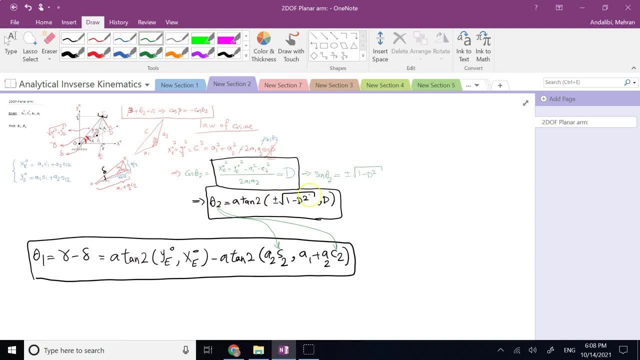 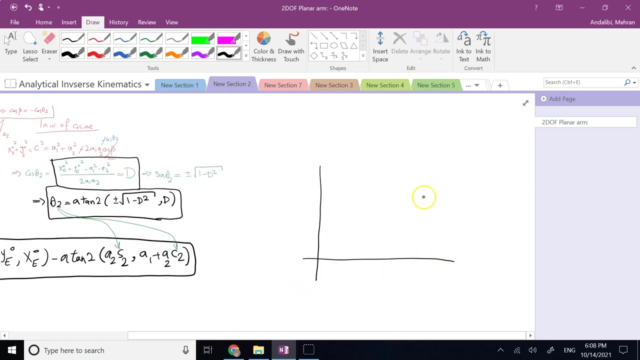 solutions: one for the positive square root, one for the negative square root. okay, and so, uh, the inverse kinematics problem in general can have two solutions. now, what are those two solutions look like? let me show you that. so, if this is the the base frame and this is a specific position, and i want to reach that point, one way to reach it is: 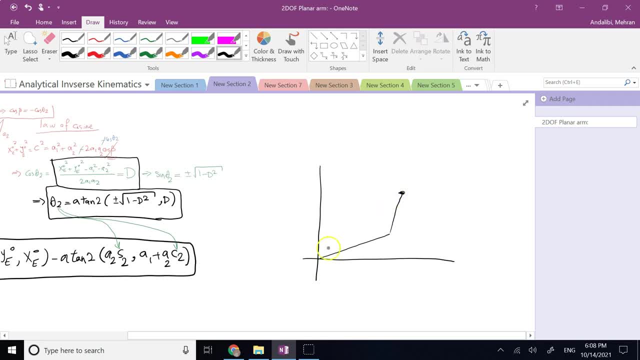 this. the other way to reach it is this. so of course the end effector orientation will be different. but here we don't care about the end effector orientation, we only care about the end effector position. so in one of the cases it will be like this and the other one it will be like that because it's rigidly attached. 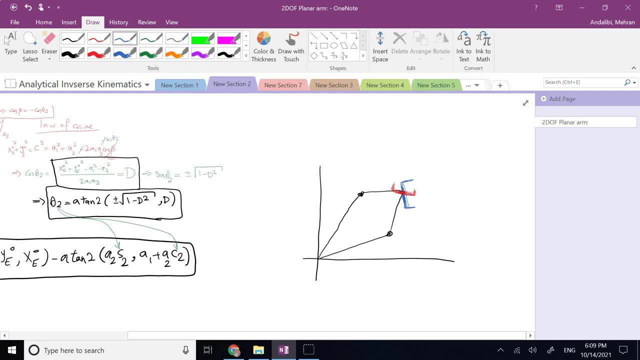 to number two, but we just need to reach that point correct. so in this case, clearly, your theta 2 is positive because it is counterclockwise, and in this case here, clearly, your theta 2 is what? negative? okay, so this condition that theta 2 is positive, we call it what? 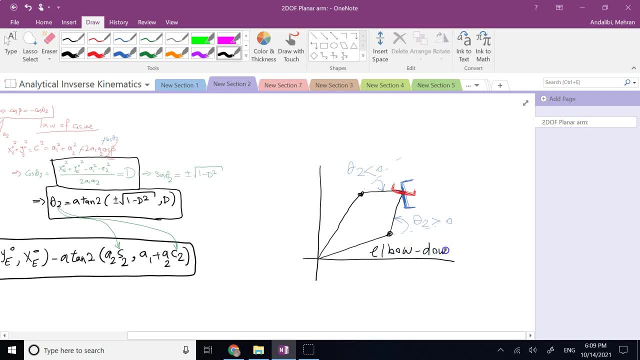 we call it elbow down, and this one we call it elbow up. so there are two separate solutions for the problem of inverse kinematics: elbow up and elbow down. now you might say: well, is there any scenario where you're going to be able to find the end effector? 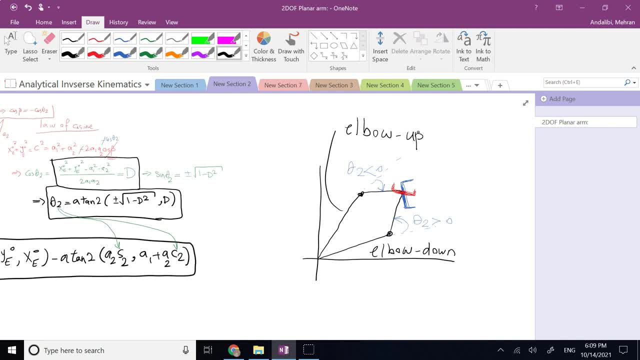 where there is no solution, or one solution. sure, When is that? Well, if this point that I'm going to reach is outside the workspace, then there will be no solution. But you might say, okay, where is the workspace, or how large is the workspace? 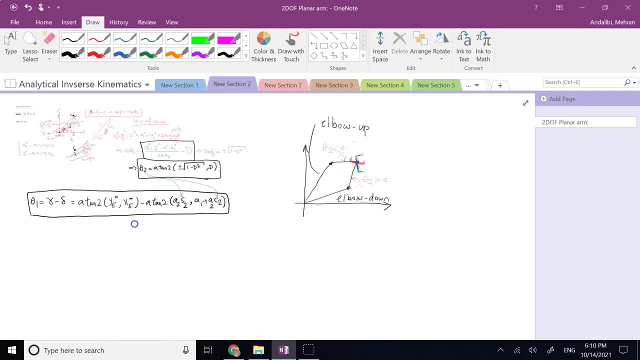 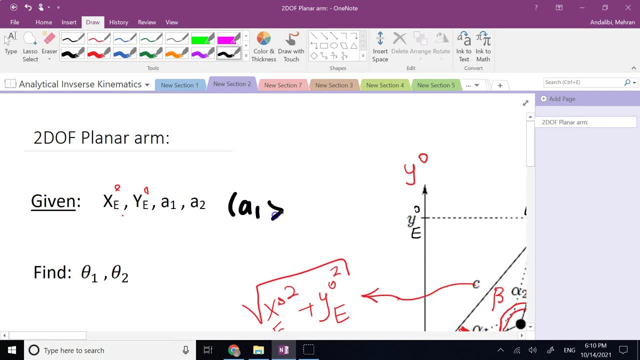 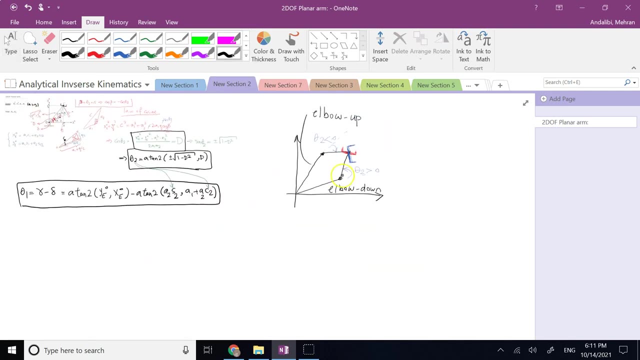 Well here, if we assume for the moment that A1 is bigger than A2.. So this A1 that we have is what Bigger than A2, then what? Then? what you will have is the maximum reach that you can have is when theta two is zero. 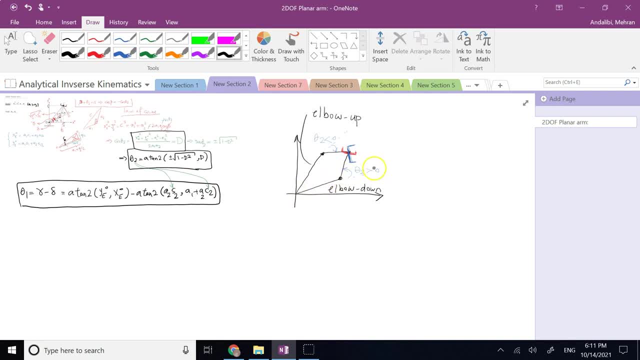 so the two members are aligned, then the maximum radial distance you can reach is A1 plus A2, and the minimum that you can reach is when member two is completely again aligned back on member one. but theta two is pi, so it is backward. 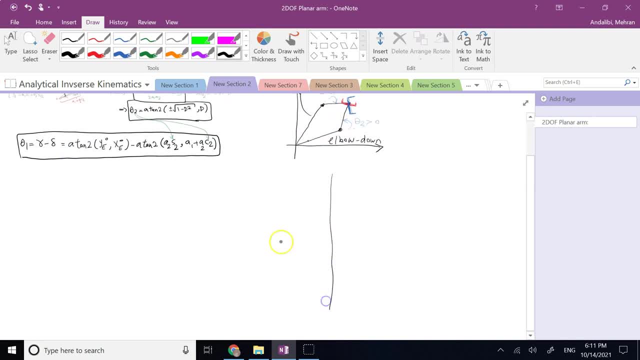 In other words here. In that case, your workspace is going to be basically a disc. Okay, so you will have a disc here and you will have another disc here, Both centered at origin, where the radius for the big guy is A1 plus A2.. 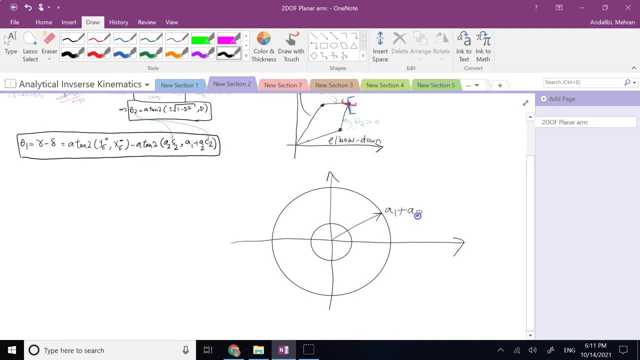 Let me show you that side. And the radius for the smaller one is A1 minus A2.. So this area here that I'm using the hatching lines, this is going to be your workspace. Okay, assuming that A1 is bigger than A2,. 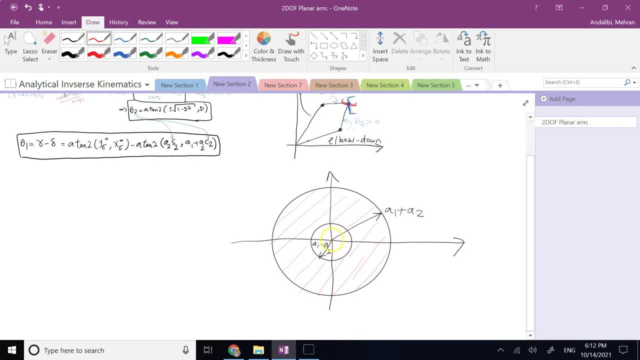 you might say: what if A1 is equal to A2, when then there is no disc? It's gonna be a solid circle. You can reach the origin as well. And if A2 is bigger than A1, then what? Then again the same problem. 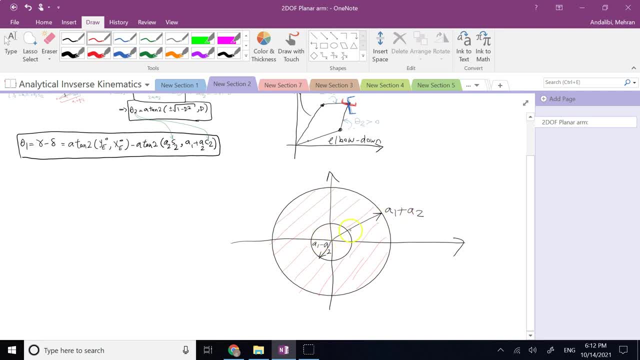 because now, if it's completely, member two is moved back and theta two becomes pi, then you will have something like this: So this is A1,, this is A2.. Again, can I reach origin? No, I cannot. So again you will have the same thing. 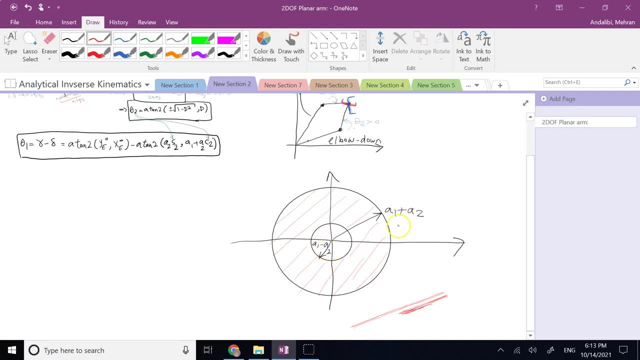 but this radius is gonna be A2 minus A1.. So as long as A1 and A2 are not the same, you will have a disc. When they are the same, then the disc will be. there will be no hole in the middle of the disc. 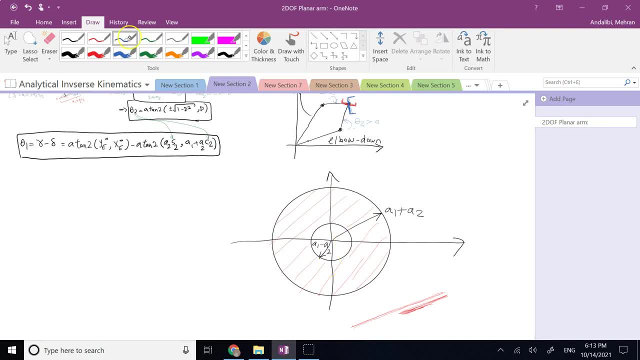 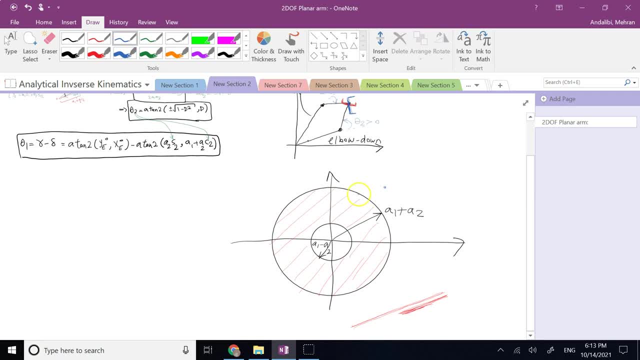 No solution, right? And what if it is on the boundary of the workspace? So what if the point I want to reach is exactly on the boundary? Then of course, here you have to make the two members completely stretched out, So theta two has to be zero. 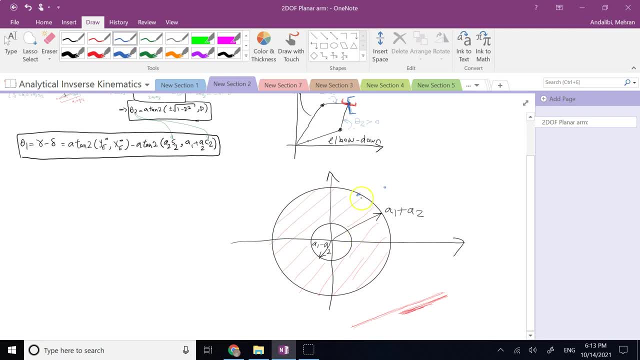 And then theta one is just given by arc tangent two of Y of n the vector and X of n the vector. okay, And the same thing here. right, That's the same thing. Theta two is pi. And again, theta one is given by: 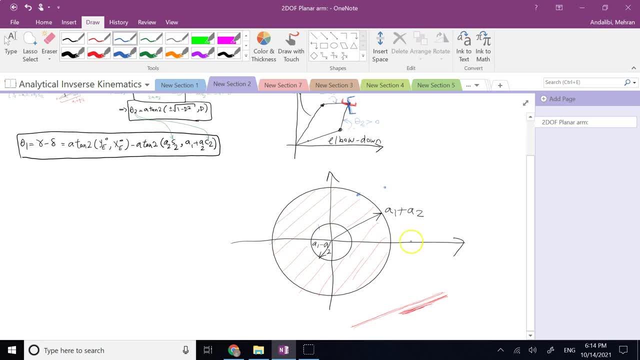 arc tangent two of Y of the n the vector and X of the n the vector. So I'll write it down for you. but just pay attention: On the boundary there is a unique solution. Outside the boundary, there is no solution. 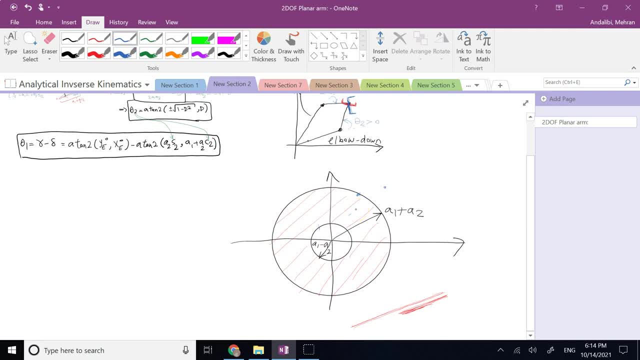 Inside the boundary there is elbow up and elbow down, And you might say: is there any case of infinitely many? Are there any solutions? Yes, there is, And that is only when a one is equal to a two. So, if a one is equal to a two, 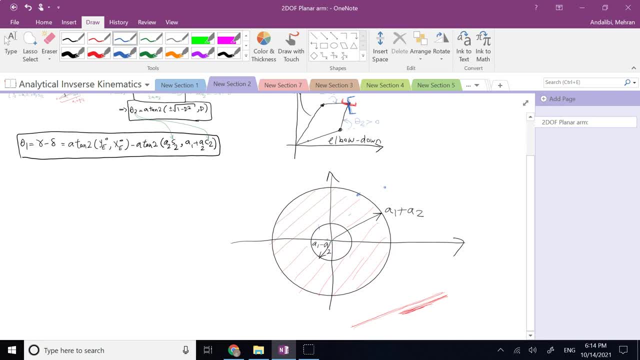 and the point that you want to reach is origin. Okay, so let me show you that If a one is what Equal to a two and the point you want to reach is origin, then what's gonna happen? So here is one of your Xs. 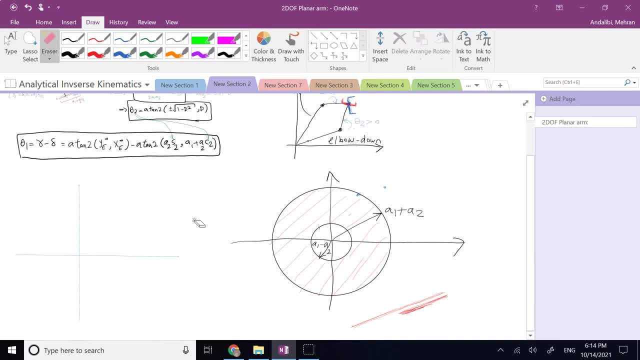 This is the other Xs, And here I have the workspace which, as I said, it is a circle centered at origin. A one is equal to a two, And you want to reach origin. Well, one member is gonna be this way. 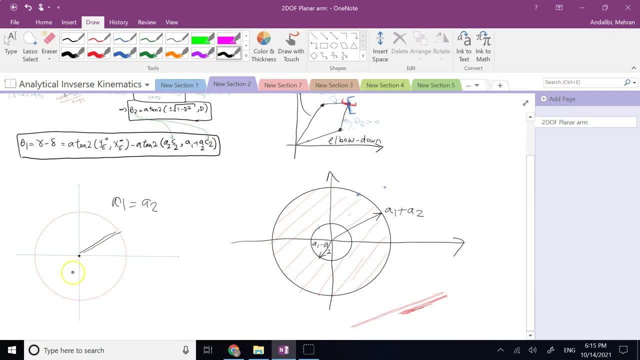 The other member is gonna be like that, So I can reach it this way. Or one member can be like this, The other member can be like that, Or it can be like this And then back like that. So in this scenario, 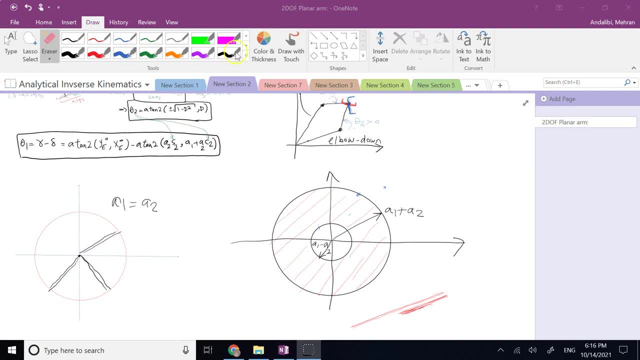 theta two is pi and theta one is what? Arbitrary. Let me write it down for you. So theta two is pi, but theta one is arbitrary, And arbitrary means what Means infinitely many solutions. So the only case is this Reaching origin, when the two members are equal size. 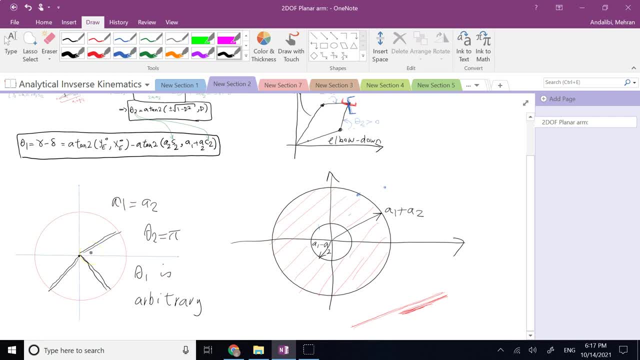 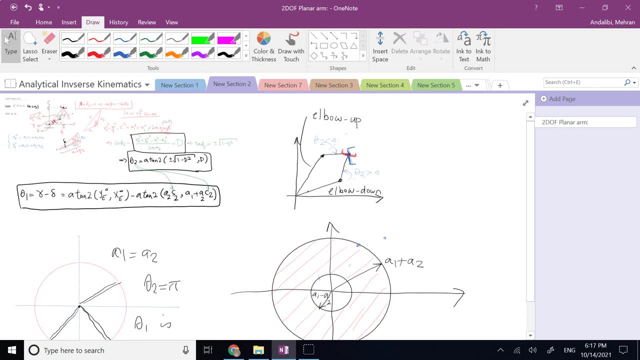 then there are infinitely many. what Solutions? Okay, So this is the overall analysis of inverse kinematics for 2DOF planar R. Now can I find the conditions mathematically for when, like let's say, I want to write a code? 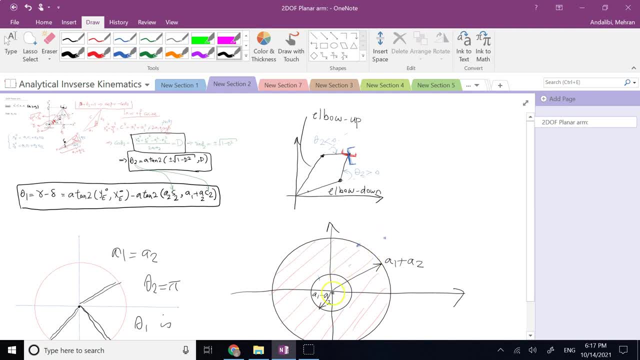 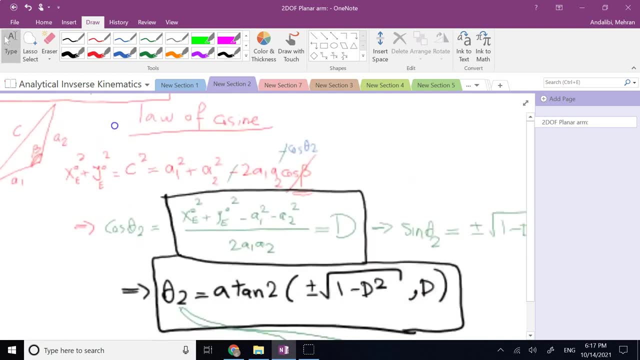 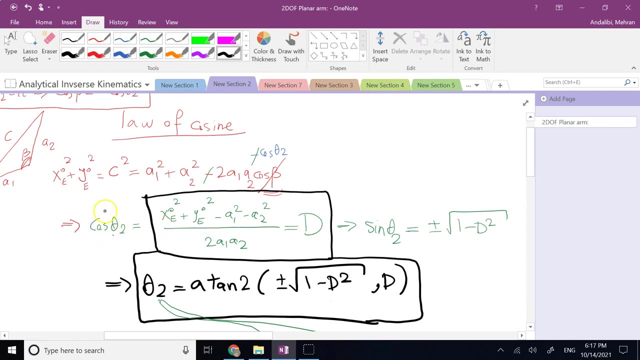 for when there is no solution, or there is what, There is a unique solution or there are two solutions. How can I find that mathematically? Well, it all goes back to this definition of d. Remember: d is cosine of theta And cosine of any angle is between negative one to one. 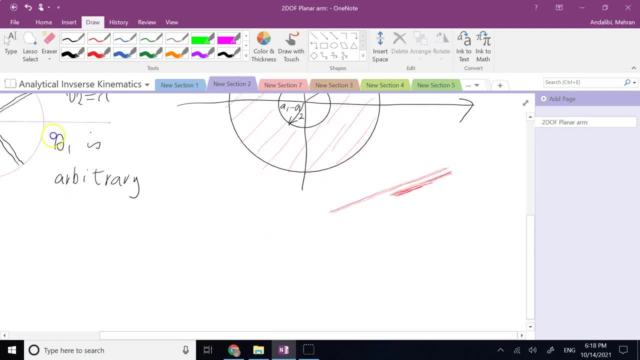 Correct. So that gives you the condition that you need. So let me write it down for you here. So remember cosine of theta two, which is equal to this ratio. It is going to be between negative one and positive one, Right, That's all you can do. 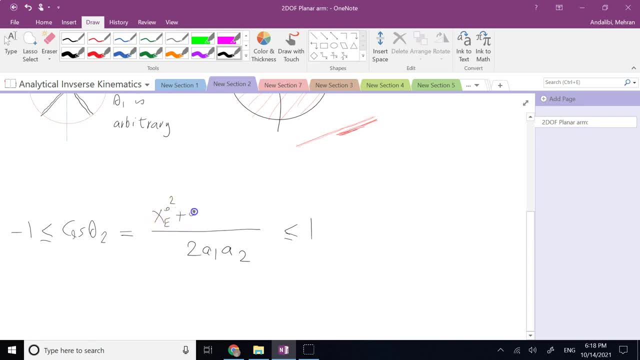 Therefore it gives you limitations on where you want to put your position of the end effector. Now, if you use the right hand side part of it and you cross multiply, you will get X of the end effector in base squared plus Y of the end effector in base squared. 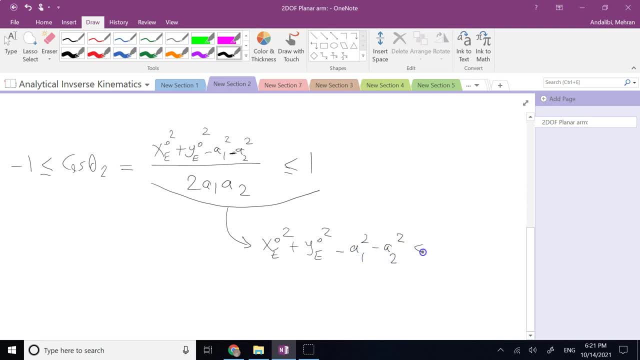 minus a one squared minus a two squared less than or equal to a one a two, Then you'll take these two negative terms and take them to the right hand side. So what you will get is this whole thing. here is going to be what. 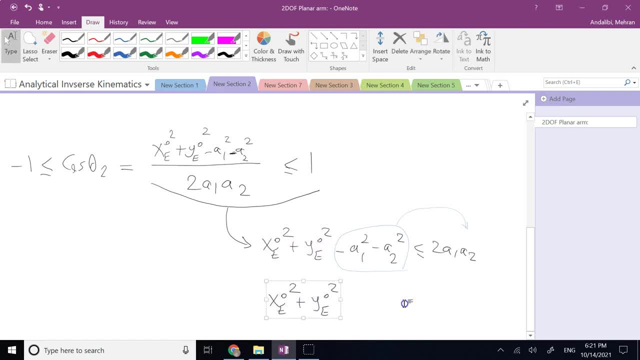 Less than or equal a one plus a two, the whole thing squared Right, Because that's what it gets: A one squared plus a two squared plus two: a one a two. On the other hand, if you do this portion of it- and you do it- 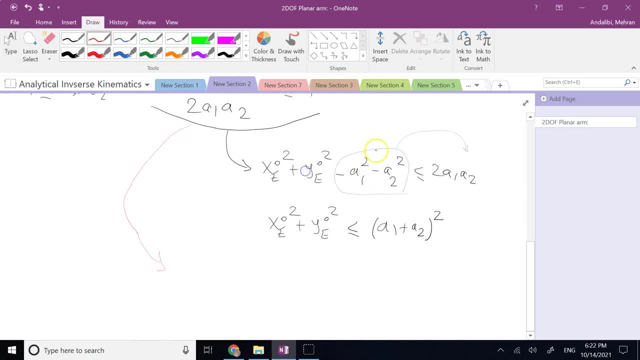 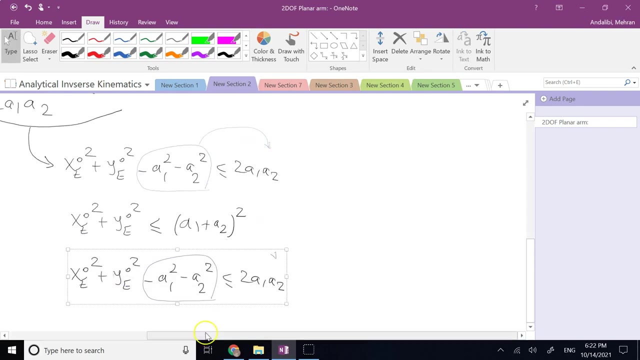 what will you get? You will get that whole thing again. It's bigger than or equal negative two a one, a two, Right. So you will get something like this: If I do it, let me bring it down here. So if you do that portion of it, 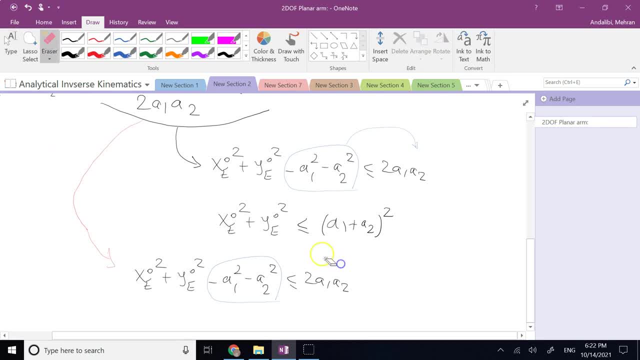 then you will get bigger than or equal negative, two times that. And again, if you take these two terms negative, take them to the other side, then you will get what You will get. your x e squared plus y e squared is bigger than or equal a one minus a two squared. 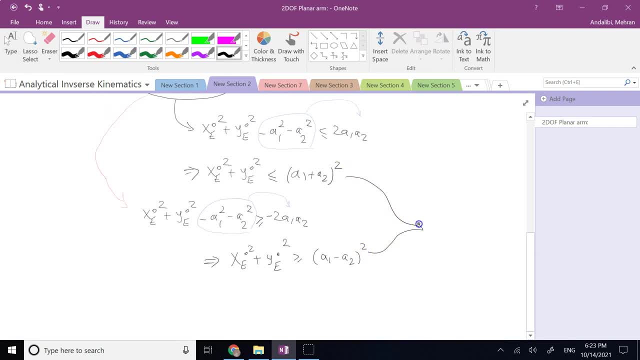 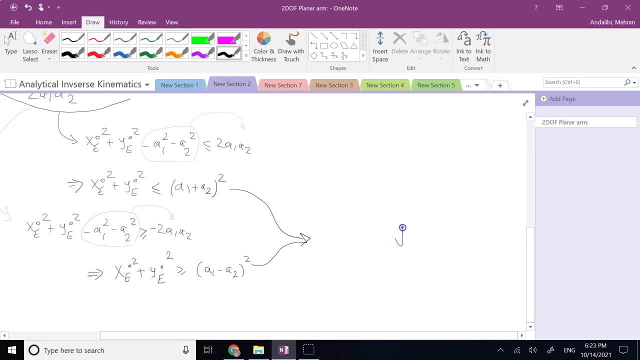 And so from these two you will get your condition. that's what the radial distance. if you take the square root, the radial distance to the end effector, which is this: a square root has to be between the two values. One of them is a one minus a two. 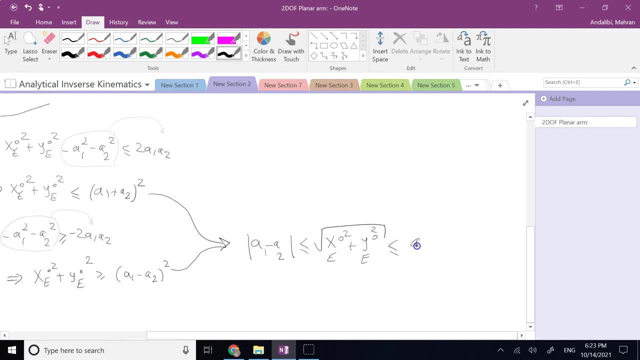 or you can say absolute value of a one minus a two And the other one is a one plus a two. So this is what This is the condition for having a square root of one minus a two. So this is what This is the condition for having a square root of one minus a two. 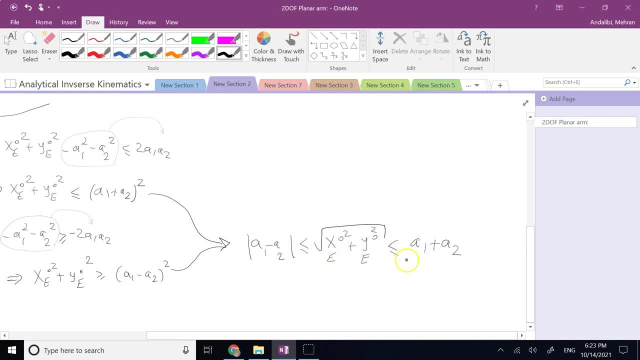 having a solution now. if the equality holds, either this one or that one means you are on the boundary. so there is one solution. if the inequality holds, then what? you have two solutions. if it's outside the range, then there is what? no solution, correct. so this is the general condition for having any. 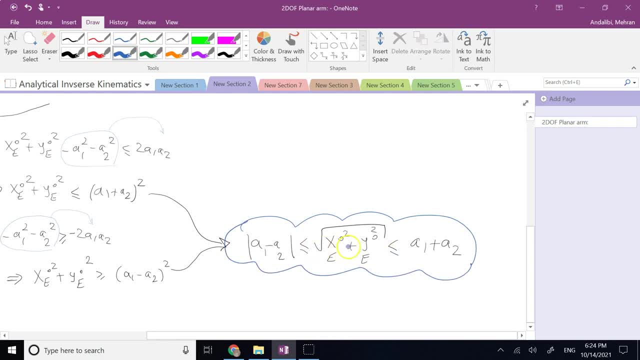 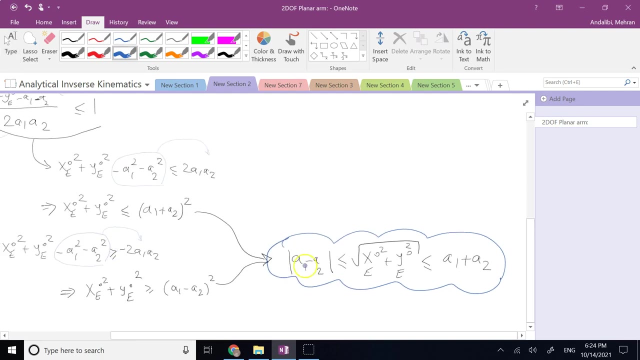 solution. but again, equality means one solution: you are on the boundary. inequality means two solutions: elbow up, elbow down. and if it's outside this range, mean there is what? no solution. okay, and the exceptional case is when a1 is equal to a2 and you want to reach origin, because then this: 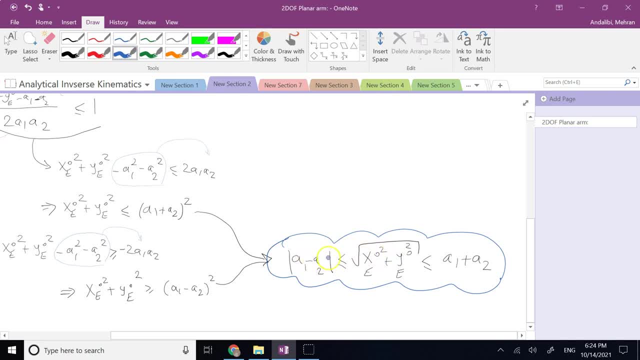 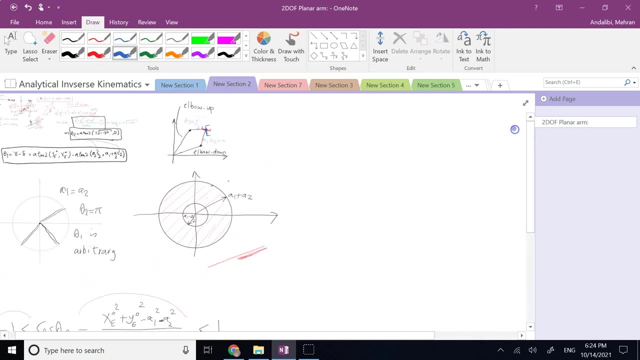 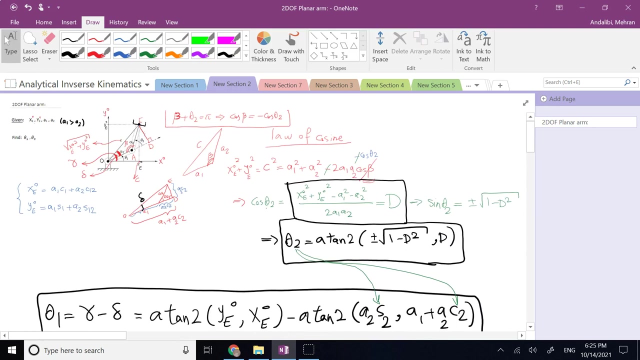 thing is going to be zero, this left hand side is going to be zero and that is going to be um 2a, and since 0 is always bigger than or equal 0, then it means theta 1 can be arbitrary. so this is how you handle the problem of what? uh? inverse kinematic for 2do planner arm. 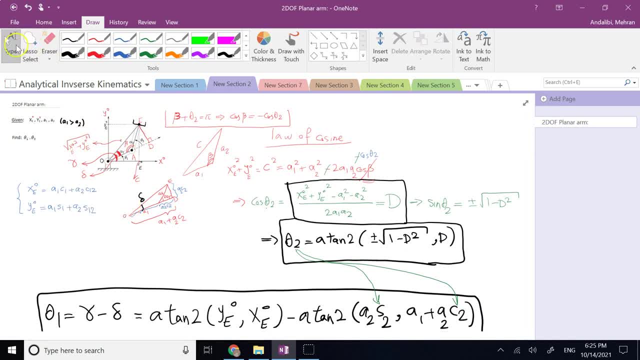 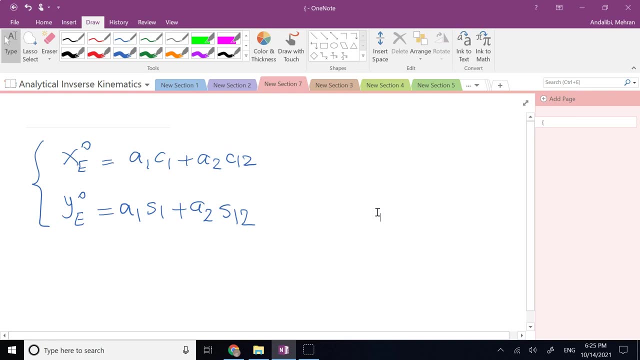 with all cases. now, is there any other way to solve this? yes, the way to do it is the um mathematical way, without any geometric help or interpretation. so, uh, since i wanted to work with trigs and be good at it, i'll show you the second way that here we solve this problem. 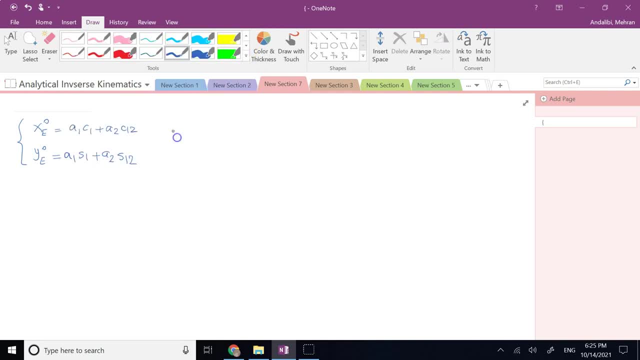 without any geometric approach, because i think it is important. so what we do here in this case, we raise each equation to the power 2.. so these are the equations of the forward kinematics. i raise each one to the power 2 and then i add them together. if i do that, i will get this guy here. 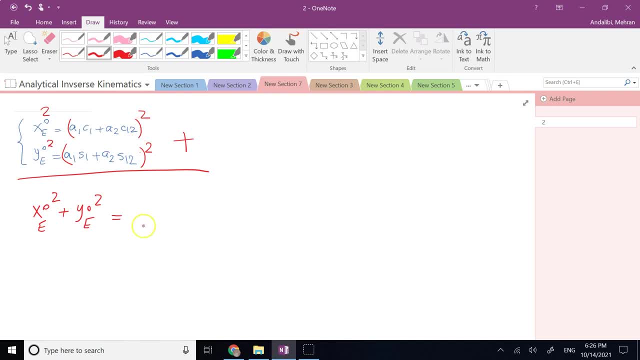 on that side it's two terms, it's a binomial. when you square it, you will get a1 squared c1 squared plus a2 squared c12 squared plus 2: a1, a2, c1, c12. that's for this guy here, and then plus. 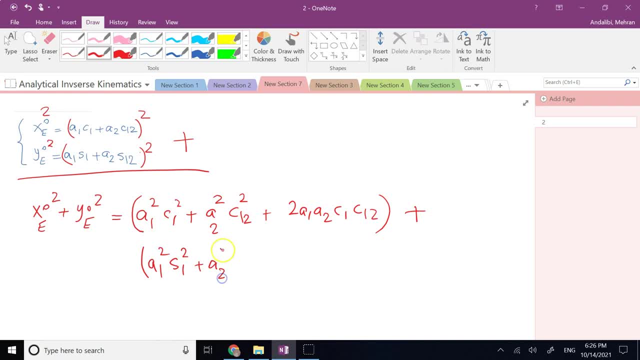 a1 squared, s1 squared, a2 squared, s12 squared, and then plus 2a1, a2, s1, s12, and now, when you add them, some of these two terms, since they have the common term a1 and a2, it's going to be s1 plus c1 squared, which is one right. so summation of these two will just give me. 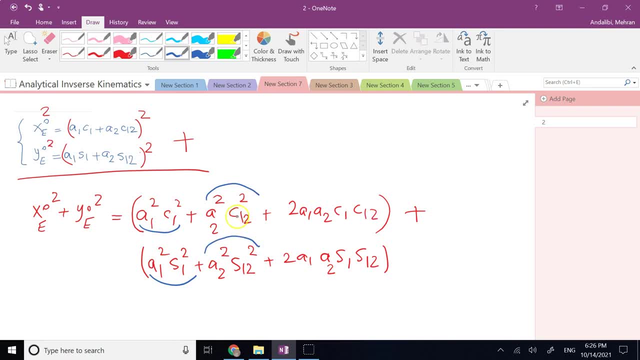 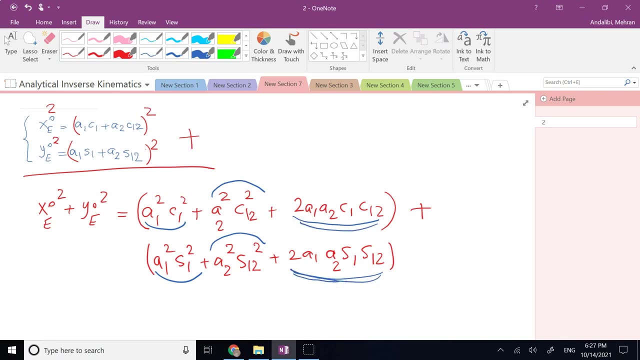 a1 squared, summation of these two terms, because again, that's c12 and s12 squared and they both share a2 squared. so summation of these two will give me a2 squared and then these two terms. if you look at them, they have the term a1, a2, which i can factor out. so if i do so, i will get x- e squared. 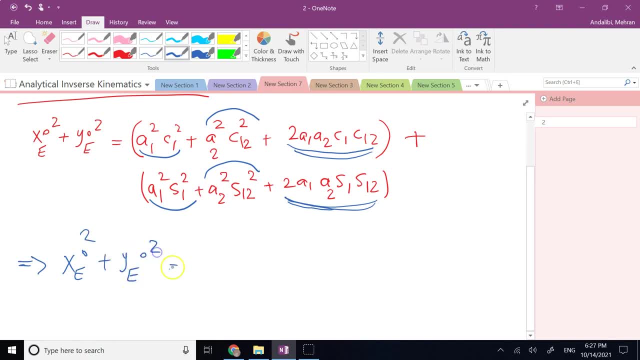 plus y e squared equals. as i said, this is going to be a 1 squared, this guy is going to be a 2 squared. those two that have 2 a 1 a 2. i factor it out, and so the result is going to be: 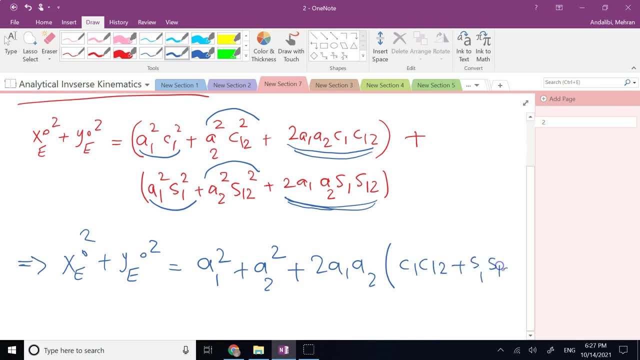 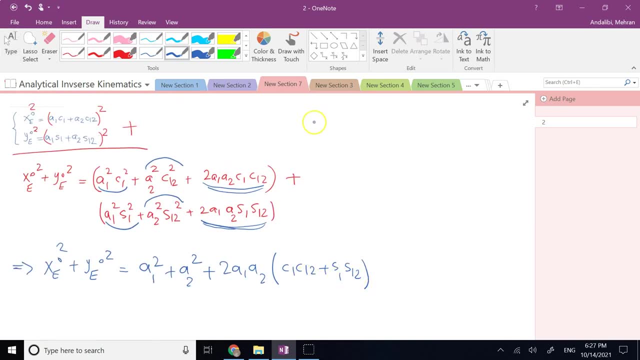 cosine 1, cosine 1, 2, plus sine 1, sine 1, 2. and now you might say: well, what is this guy? and that is where tricks come to help you. cosine of a plus b, as you know, or a minus b. in this case, cosine of a minus b is cosine a, cosine b. 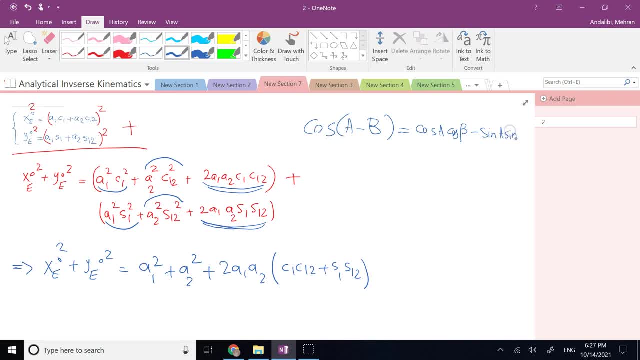 minus sine a, sine b, and that's what you have, or plus, sorry, that's what you have, product of two cosines plus product of the signs. so here, what i will do, I will do. I will consider my a to be 1, 2 and I consider my b to be 1. then a minus b is going to be one, two. 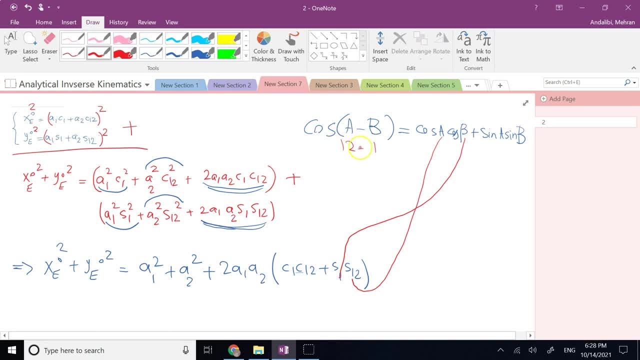 minus 1 and 1- 2. remember, that's theta 1 plus 2, this is theta 1. so the whole thing is simply going to be what theta 2. so this whole thing is what cosine of theta 2? and guess what, if you look at this, 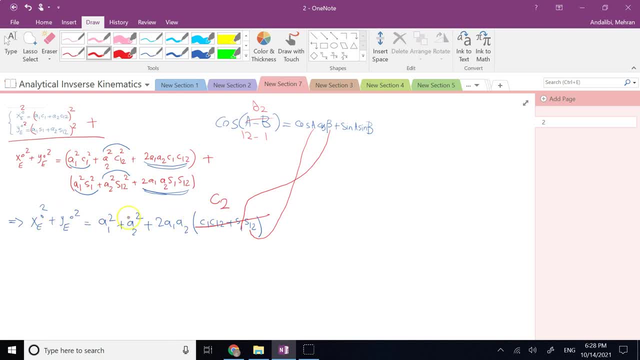 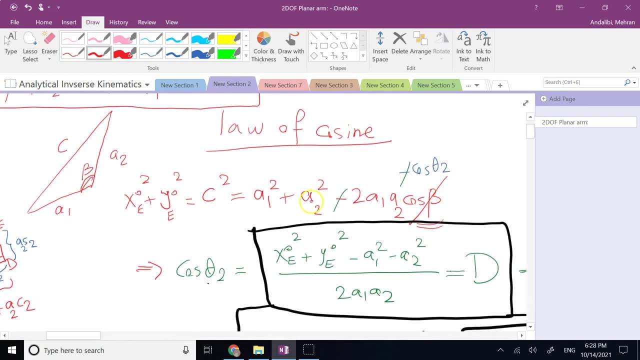 equation: x, e squared plus y squared. you have no Hope. checks at e squared is a1 squared plus a2 squared plus 2a1, a2 cosine theta 2. this is the exact same thing that we got here when we use the geometric approach. so if i define again the same d ratio, 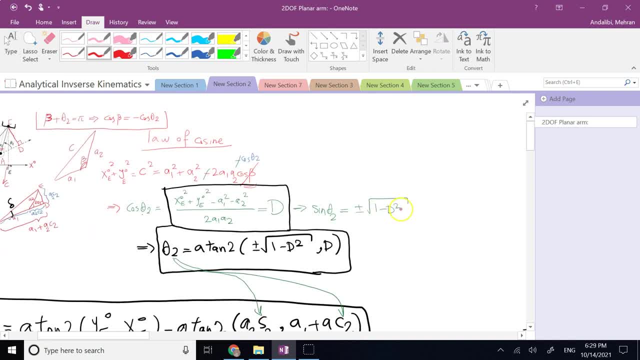 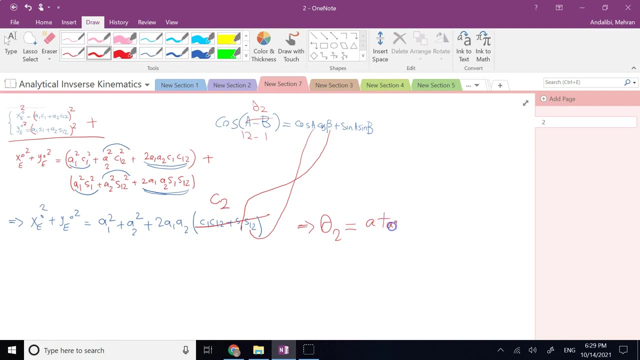 that i had, and then the plus minus square root: 1 minus d, 2 squared. that should give me the exact formula for what theta 2? so this one will lead to the exact same formula that i had. no difference. did i use any geometry? no, i did not correct. now you might say: well, can you get theta 1? 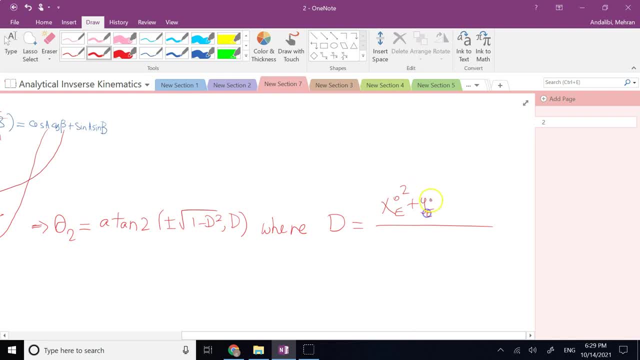 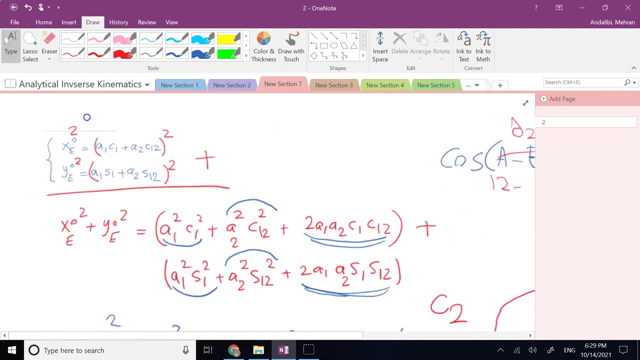 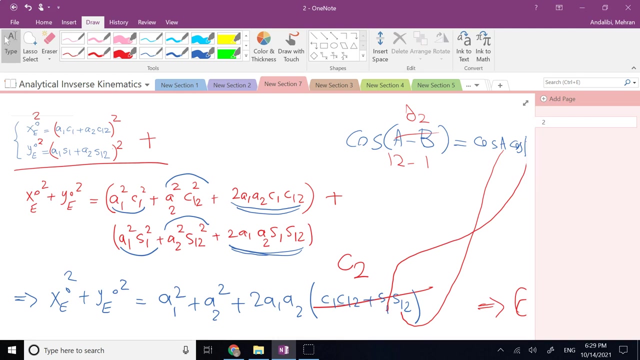 to be the same formula that you drive using geometry, without any geometrical approach. can you continue this solution and get the same theta 1 that you got last time? yes, i can. how well, let's go ahead and see how we can potentially find what theta 1 so now? what do i do now, since theta 2 here is a known value at this point, i 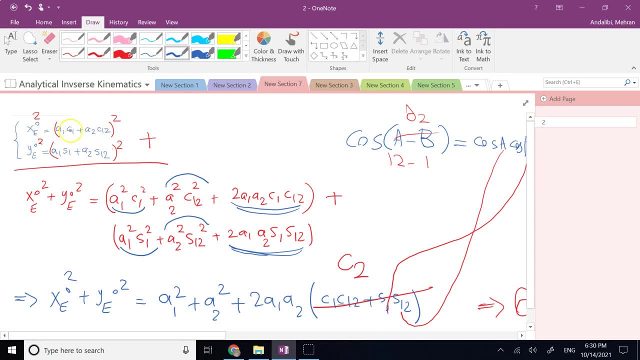 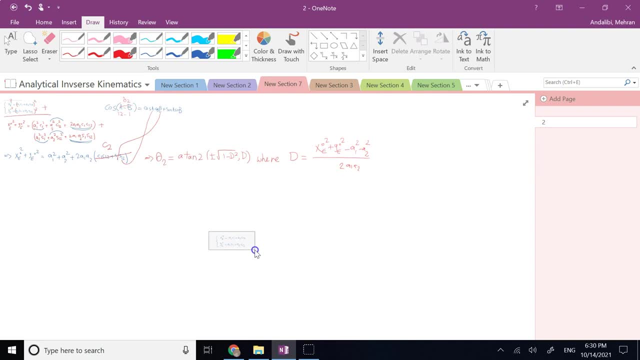 found it, then instead of adding these two and, uh, the square of them here, i do something else. so let me show you what i do next. this time i'm going to expand them, so if i do that, this is going to be a1- c1, so plus a2 and c12 means c1- c2. 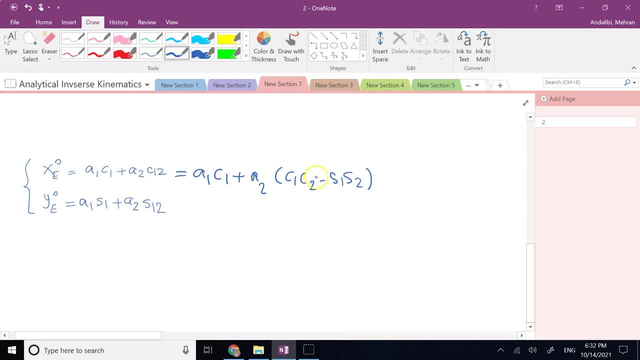 minus s1, s2, but 2 is known. when 2 is known means the c2 and s2 are known values, so i treat them as constants right now. if that's the case, then only i have a c1 term here and another c1 term here. 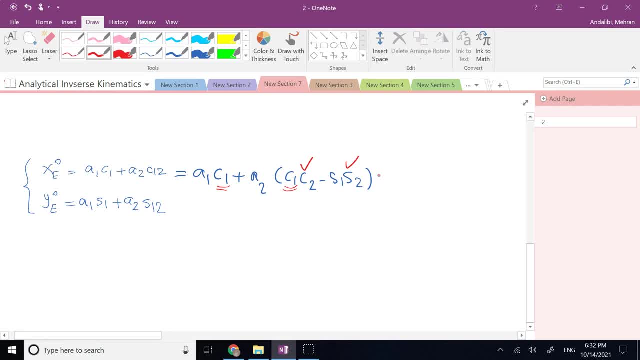 so if i factor out the um c1 term, it is going to be c1 times what here is a1. that is going to be plus a2, c2, and then this term, if i factor out s1, is going to be negative a2, s2. 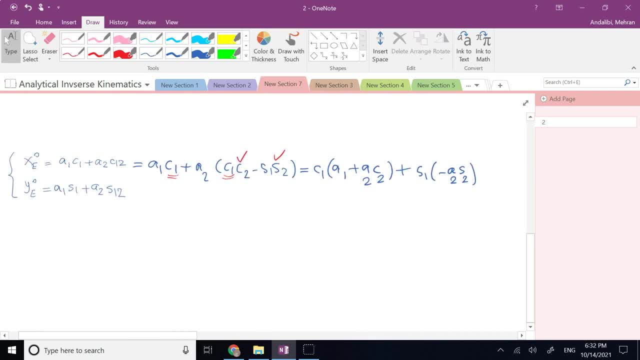 okay, that is x of e. similarly for y of e. this is going to be a1, s1 plus a2. now again, s12 is s1, c2 plus c1, s2, and again c2 and s2. i treat them as constants, if you factor out this time. 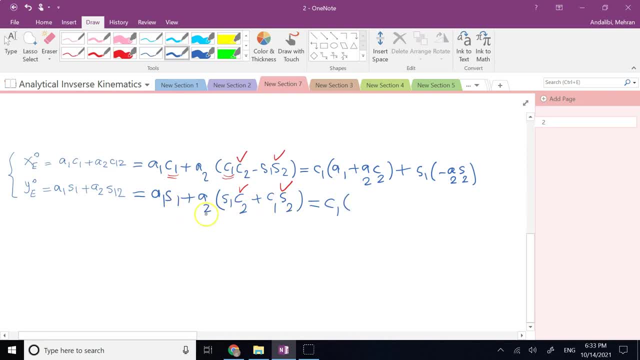 the c1 term. the coefficient of that is going to be what it's going to be: a2, s2, and this one term, if you look at it, the coefficient of it is a1, and then plus what a2, c2. good, so that is going to be a 2 by 2 set of equations where the unknowns are c1 and s1. 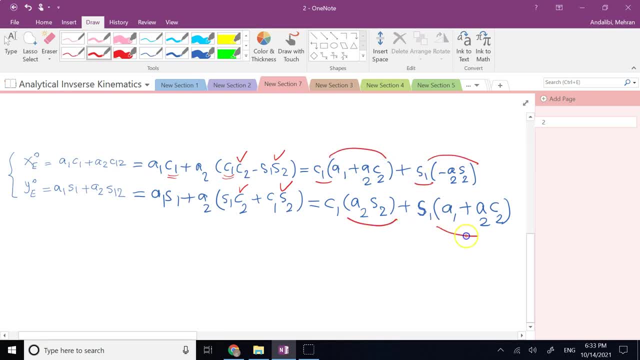 and the coefficients are these guys which are just constant at the moment, and the right hand sides are x, e and y e. so we can write it in vector format or matrix format, as x, e and y e are a coefficient matrix times what c1 and s1, and this coefficient matrix is a1 plus a2, c2. 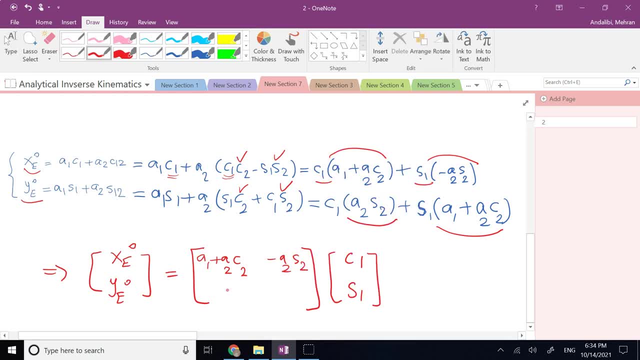 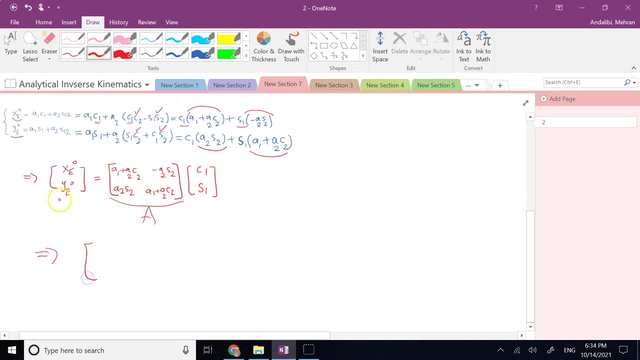 negative s, a2, s2, positive a2, s2 and again a1 plus a2, c2. if you do that, then if you call this matrix a, then and call this uh side b, then c1 and s1 are clearly a inverse times b, right? 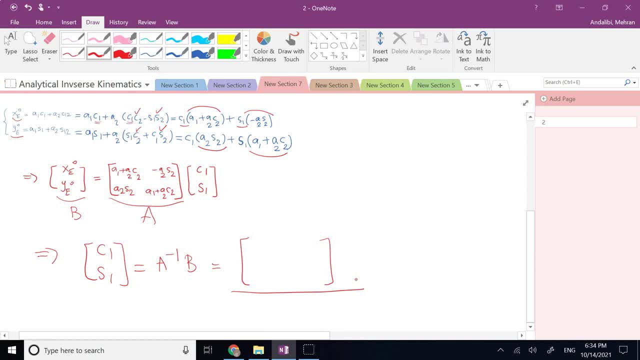 and to do that we need to um for inverse of a two by two, we swap the diagonal elements- in this case they are the same thing, so it's not going to affect anything- and then the um anti-diagonal. we negate them wherever they are. so that makes it like this: 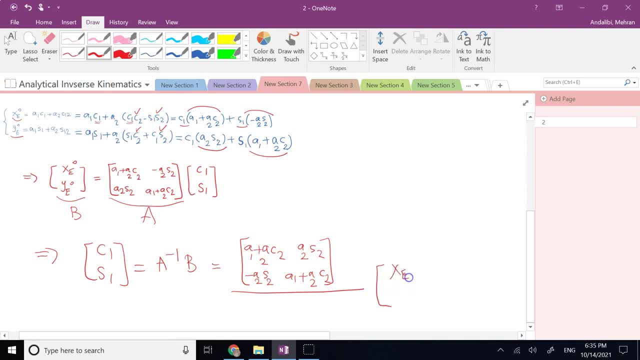 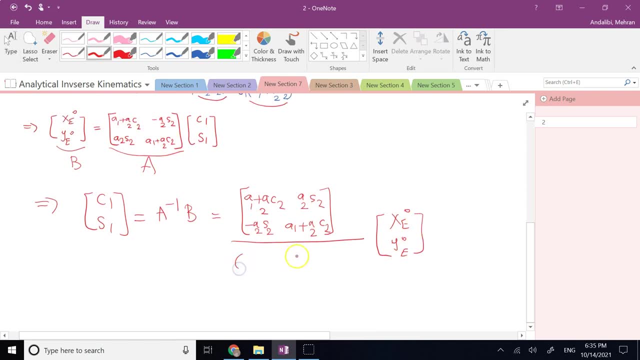 and then we divide it by the determinant of the matrix, which in this case is the product of the diagonals minus the product of the anti-diagonal. they are the same term. there is another minus here, so it's going to be make it plus, and then it's going to be: a2 squared is 2 squared. this one is that a1 plus. 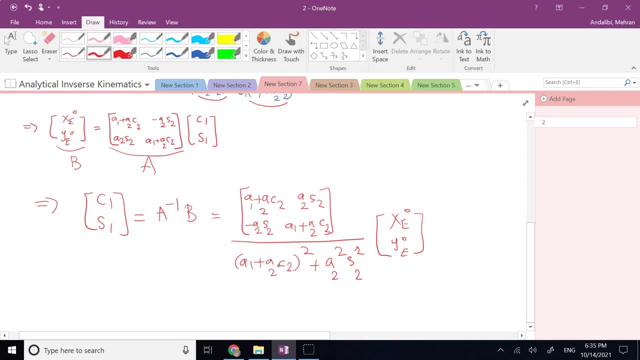 a2- c2 squared. okay, if we continue here, here, when you expand this, it's going to be a2 squared, c2 squared. summation of that with this one is just going to make it a2 squared. that's a1 squared and then you will get 2a2. 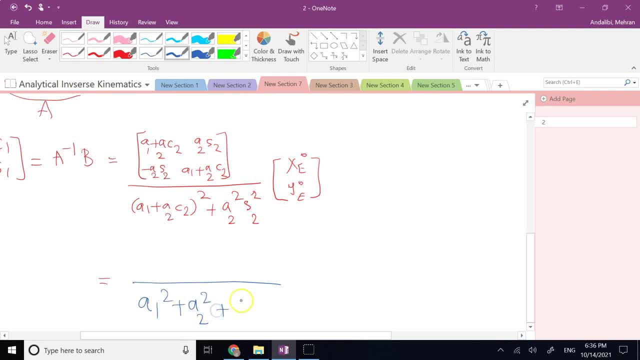 and then you will get 2a2 squared, and then you will get 2a1, a2, c2 and uh. here you will get um, the first term is going to be a1 plus a2, c2, x, e, and then plus uh, a2, s2, y, e. 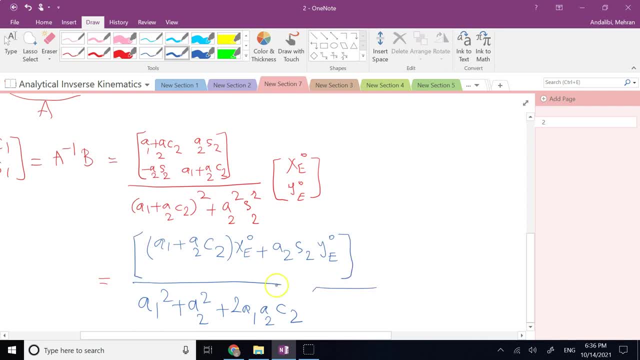 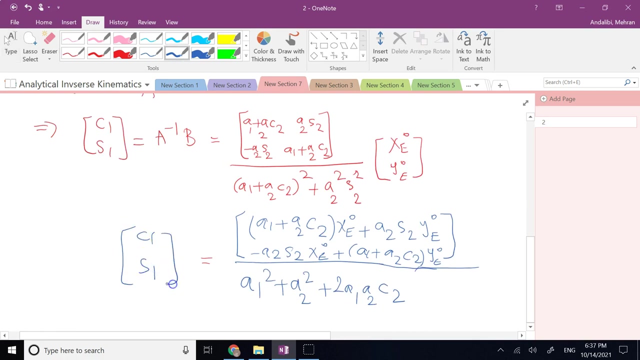 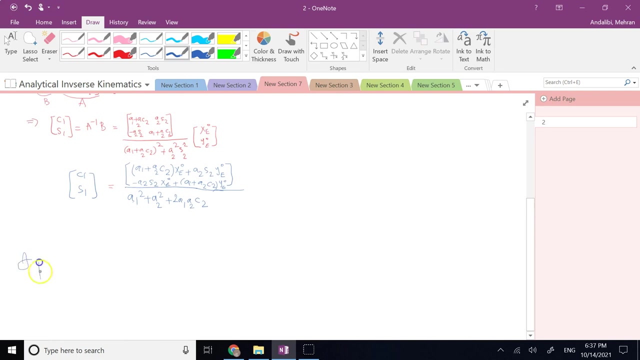 this is the first element, and the second element is going to be negative: a2, s2, x, e. then plus a1, plus a2, c2, y, e. okay, so this is going to be c1 and s1 and since they both have the same denominator when you use the arc tangent function, so theta 1. 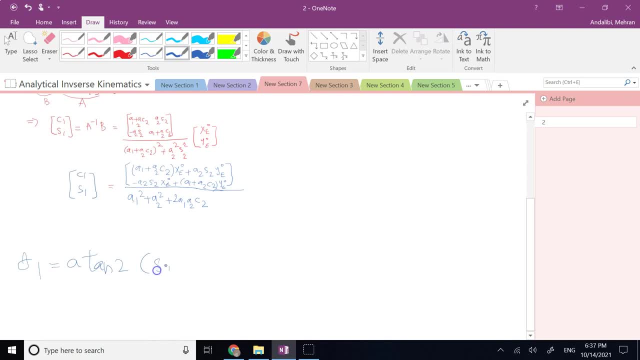 which is our tangent 2 of s1 and c1, if they both have the same denominator, and that denominator is this number here. if i neglect that because they have the same ratio, then i can just look at what these guys that they have, right, right, so it is simply can be written as arc tangent two of: 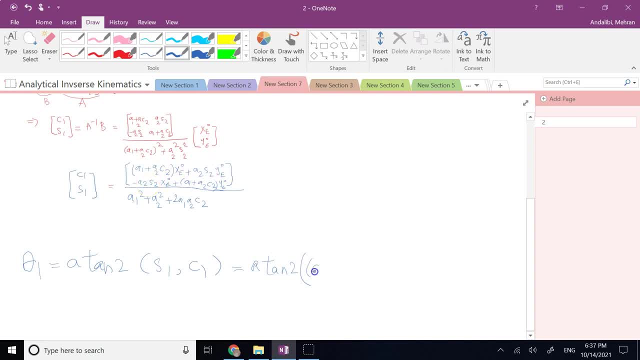 basically these guys here that i just showed you: a1 plus a2, c2, xe, right? or that's actually the sign term. so plus negative a2s2x and plus a1, plus a2c2y. That is the y term, and then I have the x term, right. 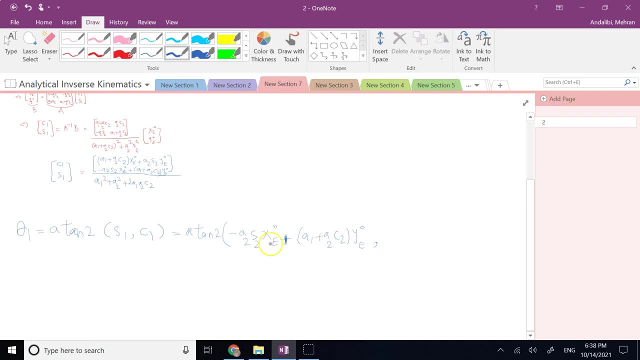 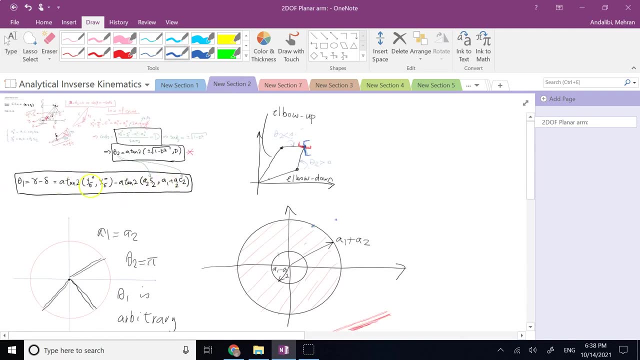 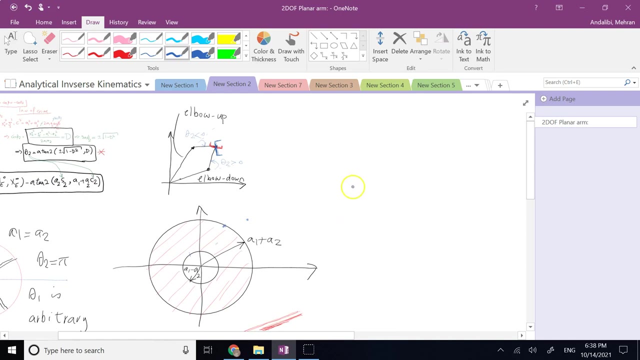 Or if I just want to show you that this one gives you the same formula as what we got here. all you need to do is to use the arctangent a minus arctangent b and, from trigonometry, if you remember, arctangent a minus arctangent b. 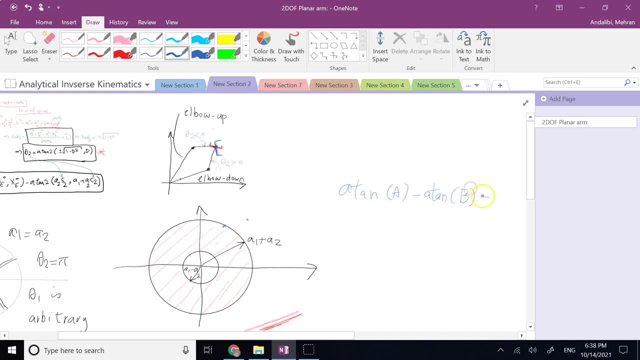 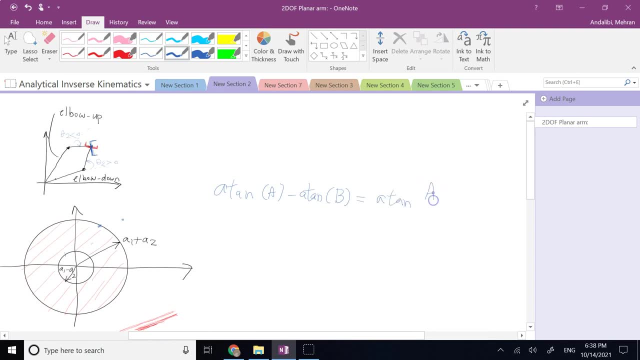 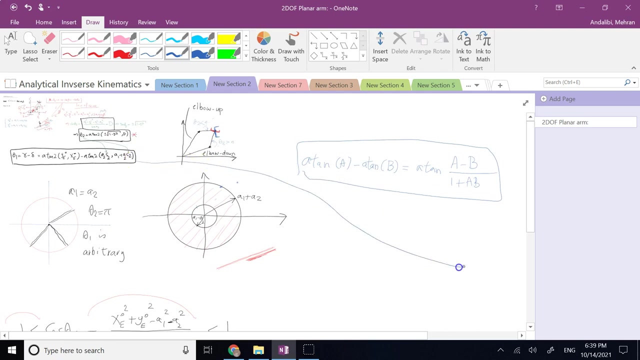 in general is what It is, arctangent of what It is going to be: a minus b, b divided by 1 plus ab. okay, So if I apply that to this formula here, right, Because this is like your a and this is like your b. 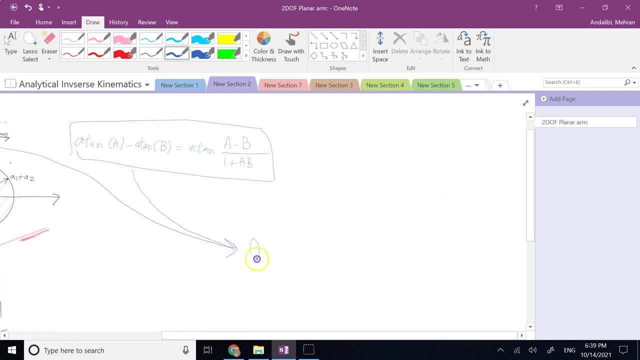 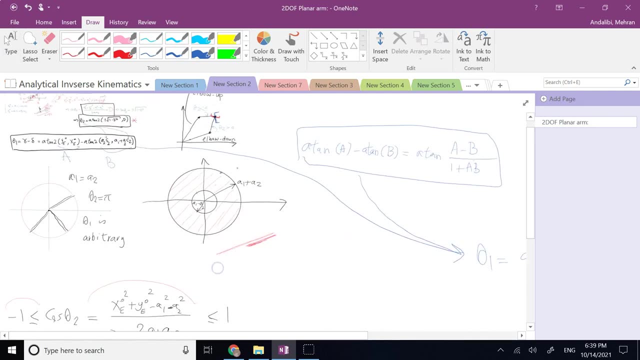 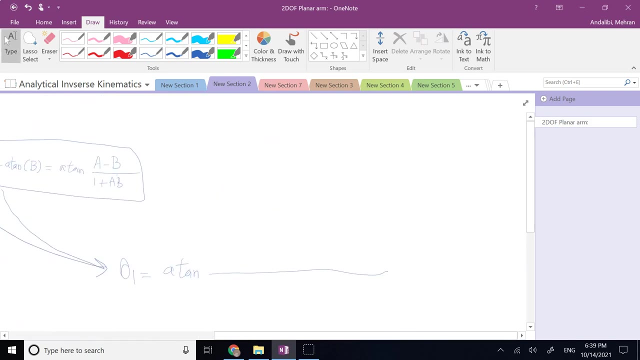 Then your theta1 is going to be what Arctangent of, As I said, a minus b, which is what, In this case, a is going to be the ratio of y over x, And then b is going to be the ratio of sine over cosine. 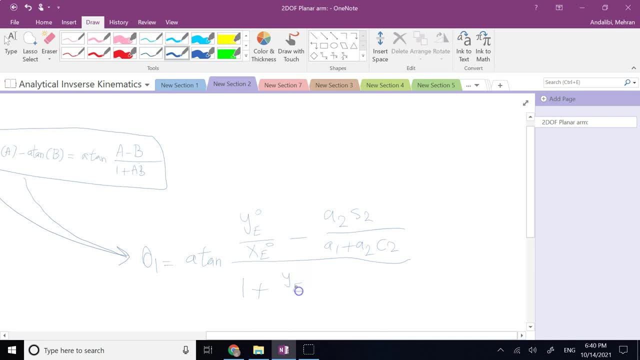 And then: 1. Plus the product of these terms. And clearly here, if you take a common denominator right, They both have the common denominator of xe times a1 plus a2c2.. Then you will get what You will get: a1 plus a2c2 times y of e minus a2s2x of e. 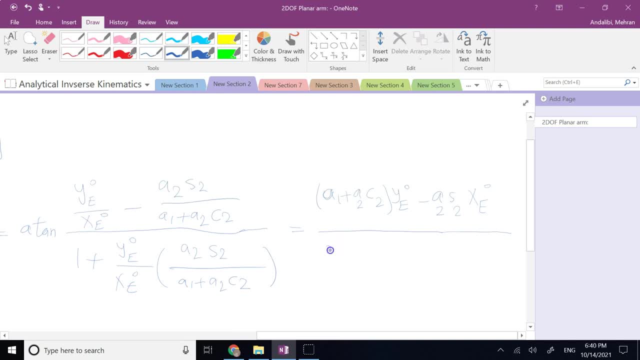 Then divided by a1 plus a2c2x, x of e plus a2s2y of e. Okay, So this is going to be your theta1,, this ratio, And, if you look, that's the exact same thing that you have here. 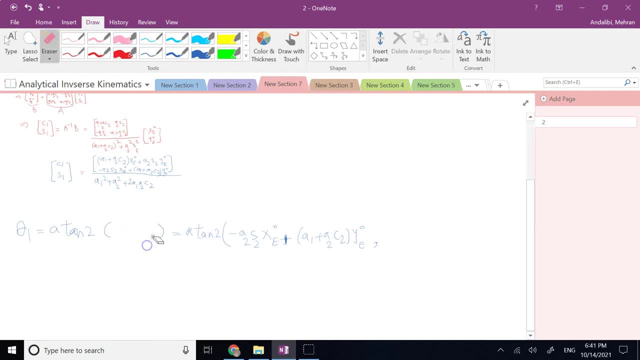 Because all you need is to just divide here, Instead of using arctangent 2, use the arctangent And if you do, If you do that, you will get the exact same thing as what you got in the other one.